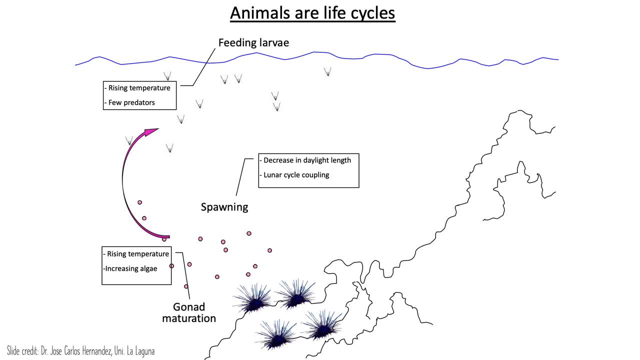 that have to gather as much food from the water column as possible, And the food for these organisms is going to be food, And the food for these organisms is going to be food, And the food for these organisms is going to be food, And the food for these organisms is going to be phytoplankton usually. 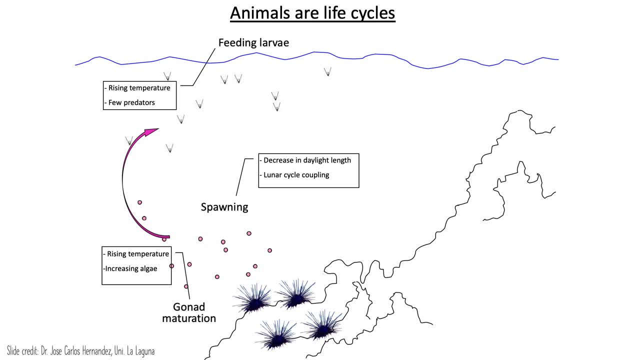 The larvae will mature and may develop through a series of different larval stages At some point then, in response to some type of cue- it could be a chemical cue, it could just be a length of time of development- type of cue. 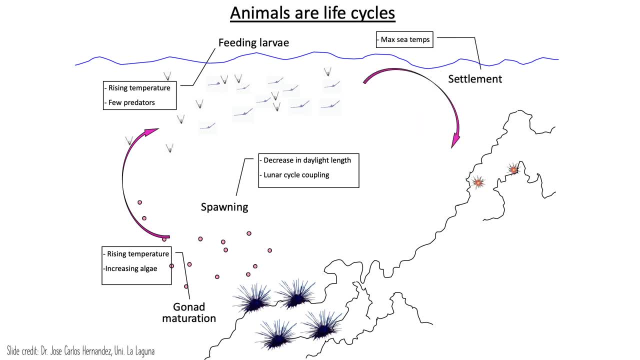 the organisms will metamorphose and settle as juveniles into the benthos, where they will begin feeding on a different food source, and ultimately, those juveniles will grow to a size such that they can then recruit into the adult habitat. How, then, do we define what is a larva or what are larvae? 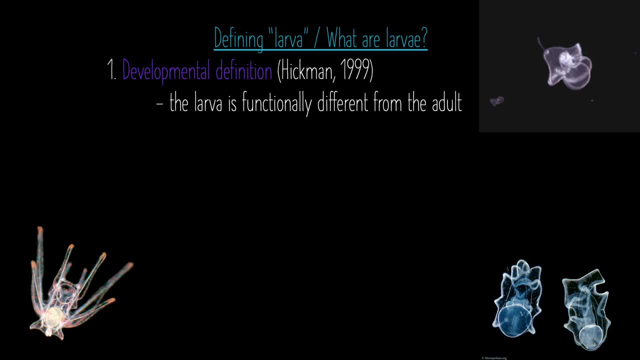 or what is a larval stage, or what are the larval stages for a particular organism. One definition is a developmental definition that was put forth by Hickman in 1999.. And this definition essentially states that the larva is functionally different from the adult. 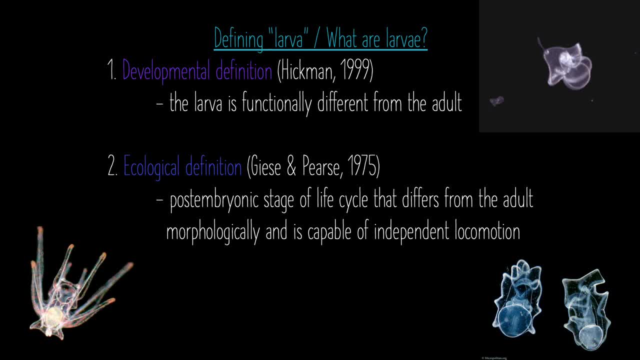 Another definition, an ecological one in this case, was put forth by Giese and Peirce in 1975. And this definition states that the larva is the post-embryonic stage of the life cycle that differs from the adult morphologically and is capable of independent locomotion. 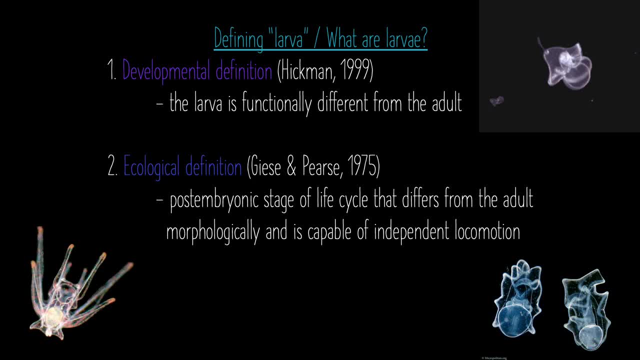 If we put these two definitions together, we essentially find that the larva, or the larval stage, is the stage of the life cycle that differs from the adult both morphologically and morphologically And functionally, and is capable of its own independent locomotion. 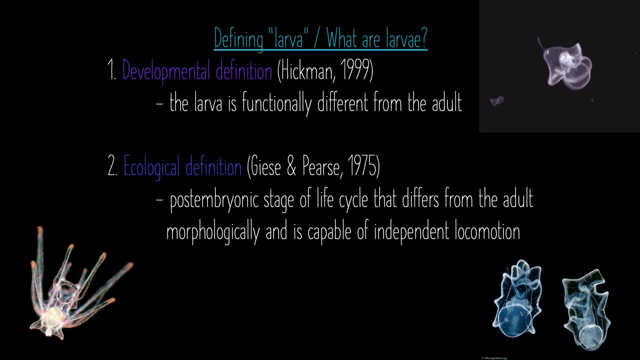 In some cases, the larvae of many organisms were given their own species names hundreds of years ago because people didn't realize that the larvae of a particular organism was a unique part of the life cycle. They actually thought that it was a different type of organism, and so it got its own species name. 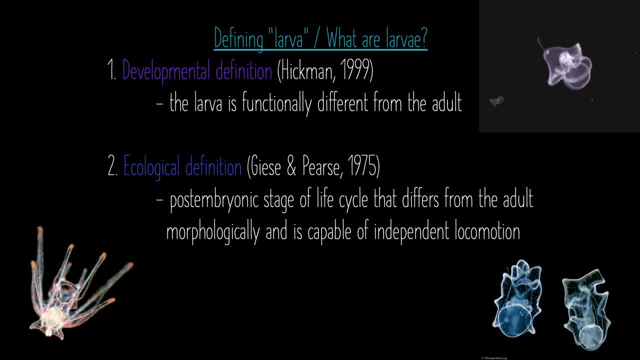 Most of these species names of larvae have fallen by the wayside, but it's still sort of an interesting bit of history to think about this idea that in one at one time, larvae were thought to be independent organisms that were separate and unique from other organisms for which we only knew the adult forms. 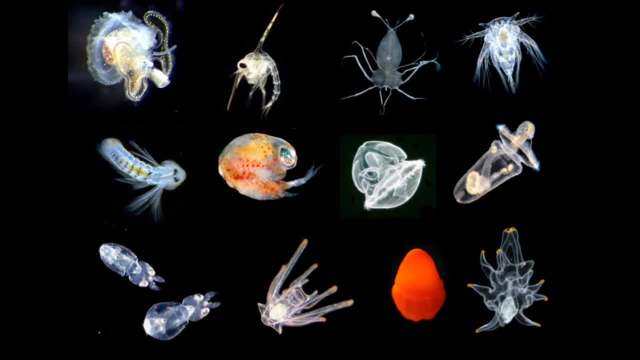 And I think one can appreciate how truly unique and diverse and beautiful the larval stages of many marine organisms are when you see them all depicted on a slide such as this. Now, this is by no means all of the larval forms that exist out in the ocean. 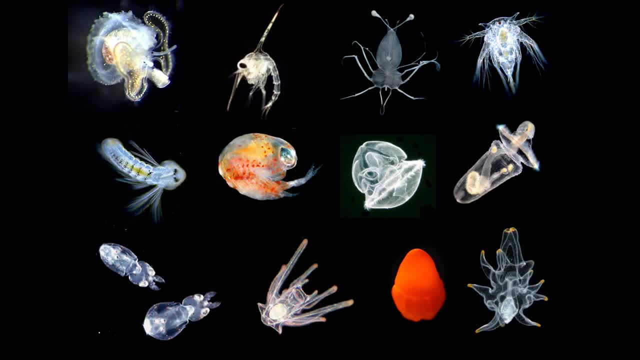 This is just but a handful, but I do have depicted here the larval stages of diverse organisms such as snails, lobsters, barnacles, annelid worms, different echinoderms such as sea urchins and sea stars. 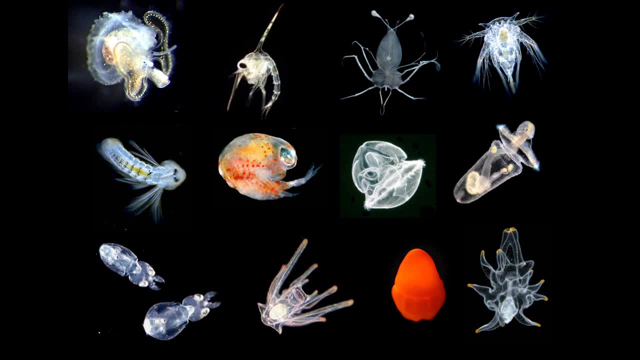 And in all cases, it's important that we understand that larvae are not just organisms that live on the surface. We understand that larvae are very important stages in the life histories of many marine organisms, because many marine organisms have this microscopic, long-lived, free-living larval stage that floats around in the water for days to weeks before settling and taking up an adult existence. 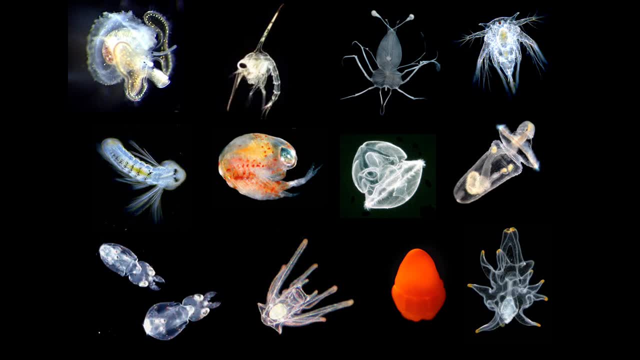 They're very diverse in terms of their morphology and function, even within closely related organisms. So, for example, I've highlighted two larval stages of larval species that are very diverse in terms of their morphology and function, even within closely related organisms. 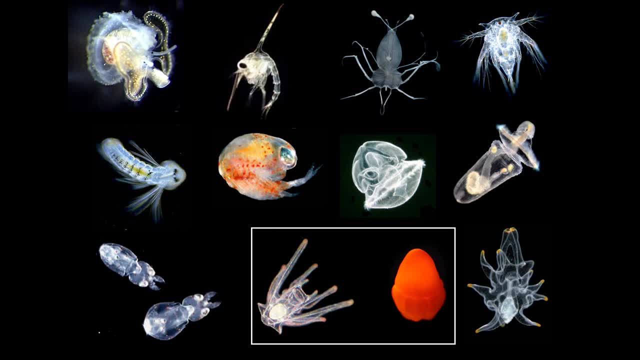 Here on the left is a feeding larval stage for a sea urchin, and on the right is a non-feeding larval stage for a different species of sea urchin. In both cases, these larvae are fully formed, and the difference is that for the one on the left 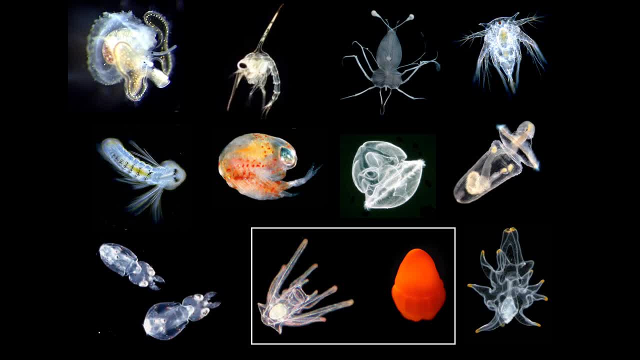 the larva has to feed on phytoplankton food in order to grow and mature, whereas the one on the right does not have to feed. So even within taxa you can find, even within Cnet компании's naar scoop. 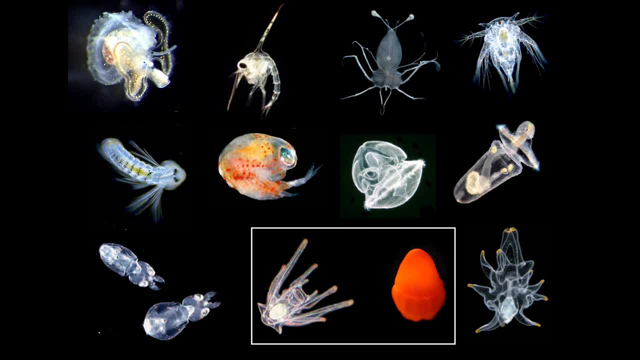 Even within closely related taxa, you can find very different forms of larvae, and the life cycles will reflect the differences that you see. If we can understand how larvae- and, by proxy, also the eggs and the juveniles of marine organisms- interact with their current environment, we can learn more about the life history of 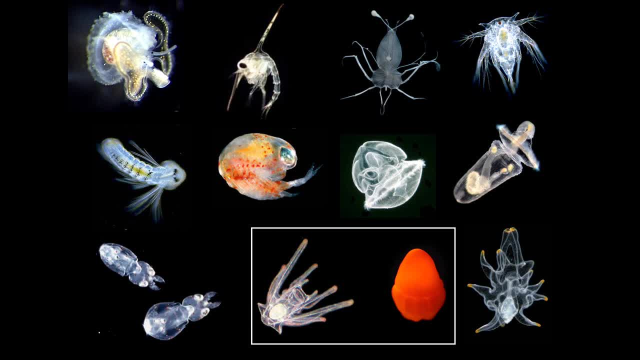 the organism, we can learn more about the dynamics of populations, and we can also understand the evolution of body form and function. Larval biology has grown to include examinations or studies that include genetics, that include ecological interactions, that examine the sizes and distribution of populations, and 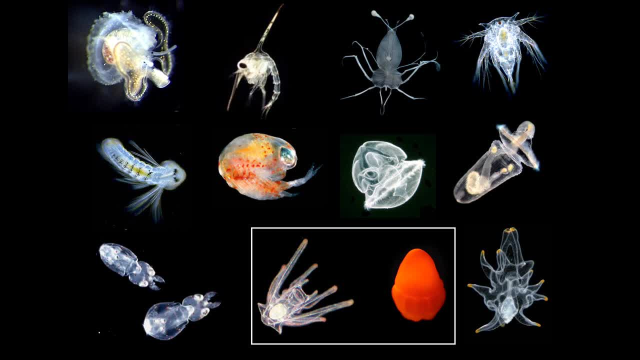 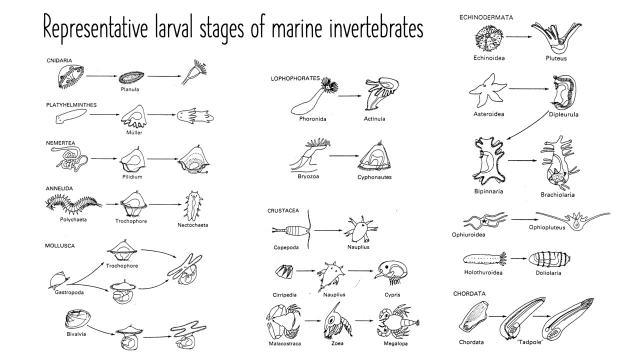 also the evolution of the organisms as a whole. So they're very important stages to understand if you really want to understand the sort of the breadth of how an organism functions. Within many different taxa, the larval stages have been given their own unique identifying. 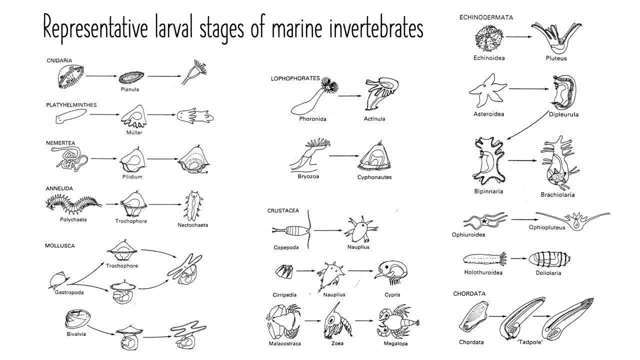 names. So, for example, in the top right of this slide we see the echinoderms depicted, and the first one there is a sea urchin, Echinoidea, and that is the adult, and to the right is the larval stage. 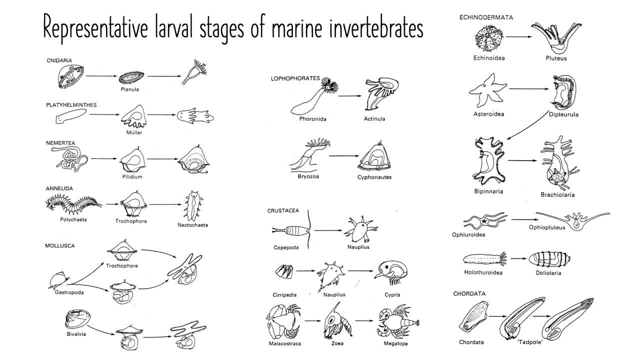 It is a pluteus larval. If you step down one organism, we have a sea star Asteroidea, that's the adult. and note that you know, in some cases sea stars will develop through three different larval stages, Not for every sea star, but for some. 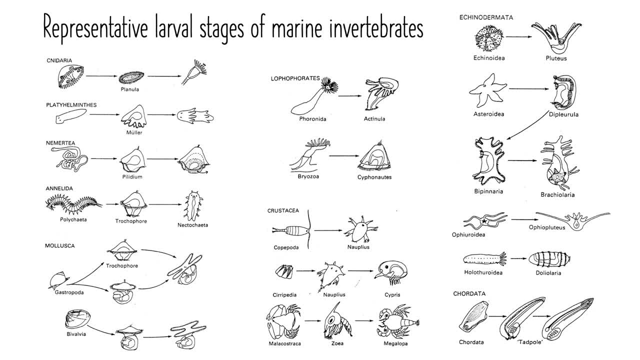 Some may only have one, some may have two, some may have three different types, But each of those different types has been given its own name. so we have a Diplurula larva, A Bipenaria larva and a Brachyolaria larva. 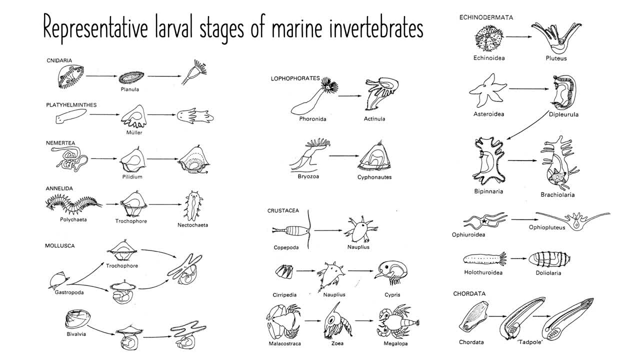 If we look over to the left of the slide, maybe about halfway down, you see the term Annelida and there is a worm that's depicted underneath it. The worm has a very unique larval form. it is called a trochophore and you see that. 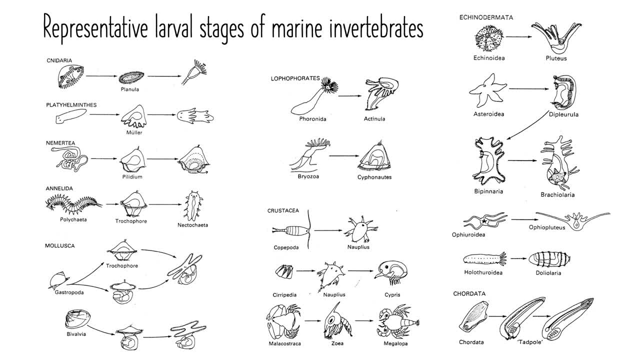 right to the right of the annelid Polychaeta and in some cases the trochophore larva will develop into a subsequent larval stage called a Nectochaeta. So appreciate here the diversity of larval forms and note that within given taxa there 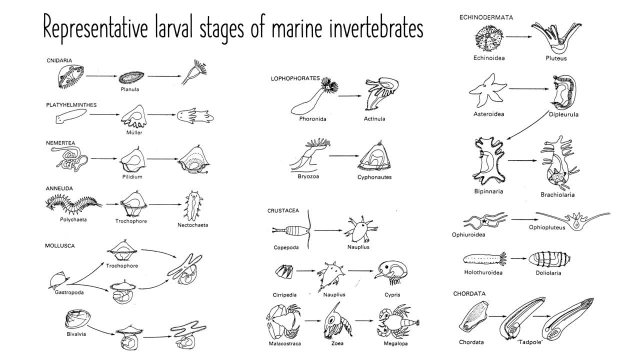 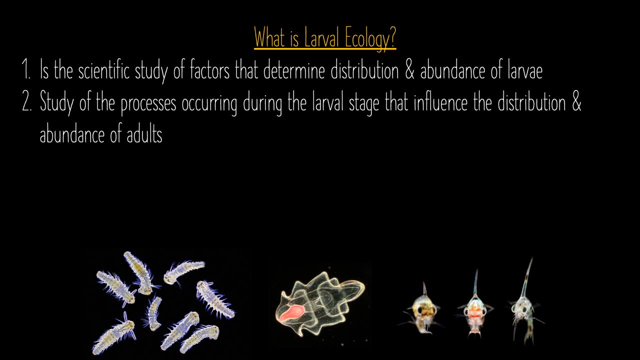 are characteristic larval forms or types that develop or are found in those particular organisms. What, then, is larval ecology? We know now what a larva is. What is larval ecology? Well, it is the scientific study of factors that determine the distribution and abundance. 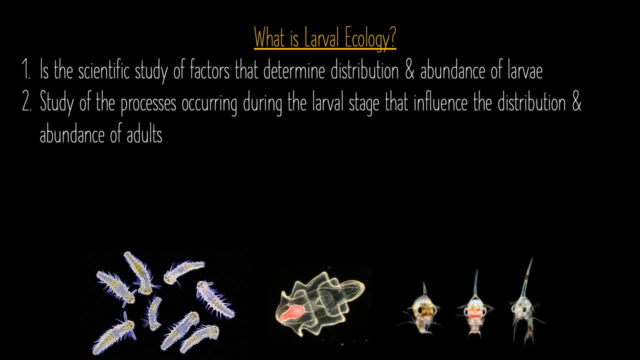 of larvae. It's also the study of processes, or of the processes that occur during the larval stage, that influence the distribution and abundance of the adults. So if you're really interested in the understanding how the organism- in this case the larva- functions, 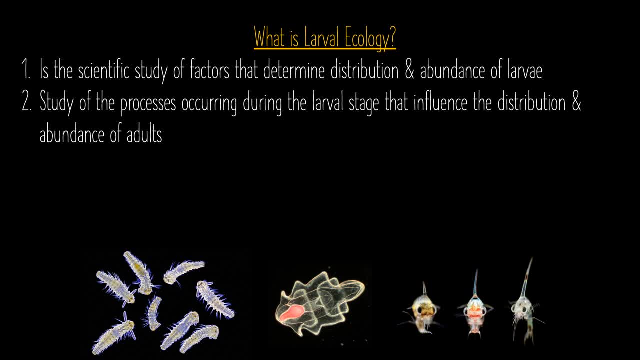 within its environment, then you are studying larval ecology. That used to be a very kind of all-encompassing term, though, And now the field has broadened to include not only ecology or environmental interactions, but also physiology, examinations of gene expression, ecotoxicological types of studies. 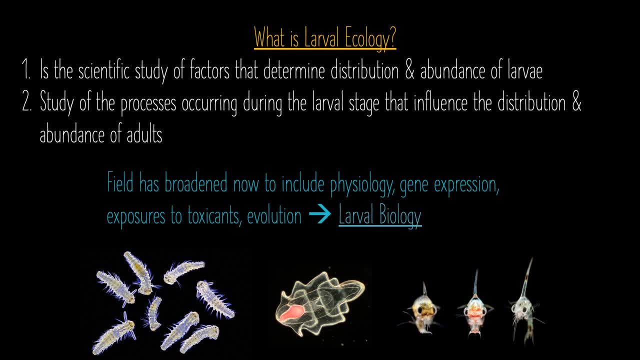 where an organism is exposed to either toxicants or physical pollutants like plastic pollution, microplastics, and then also studies about the evolution of organisms, And if you include all of those different approaches, then really you're going to be able to understand what a larva is. 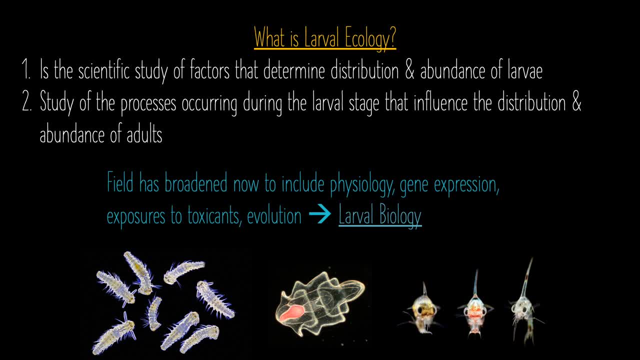 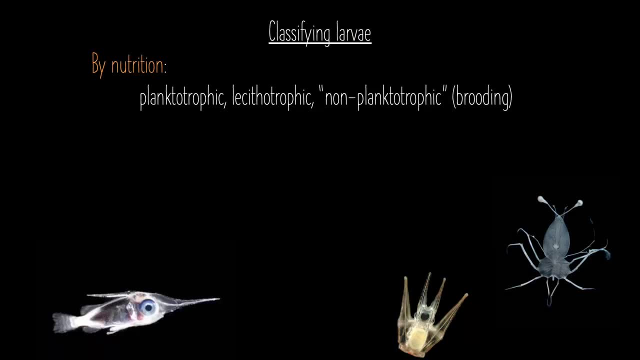 And really the field is better defined by calling it larval biology, And that's the way that we think of it nowadays. How can we classify larvae? One way we can do this is by thinking more about their sources of nutrition, or what do they feed on. 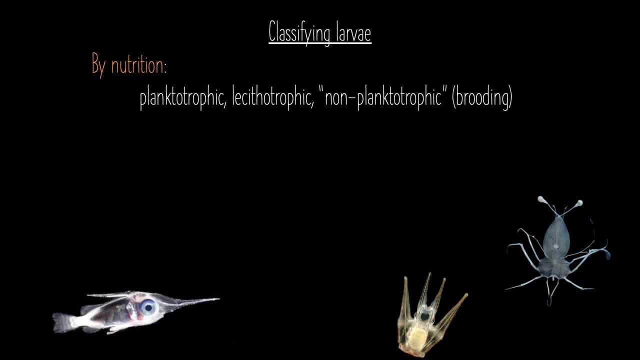 Where do they get their energy, And we have some specialized terms that refer to where their nutrition comes from. The first term here is planktotrophic and if we break that term down, the first part is plankto, which refers to plankton, and the second part is trophic, which is a term. 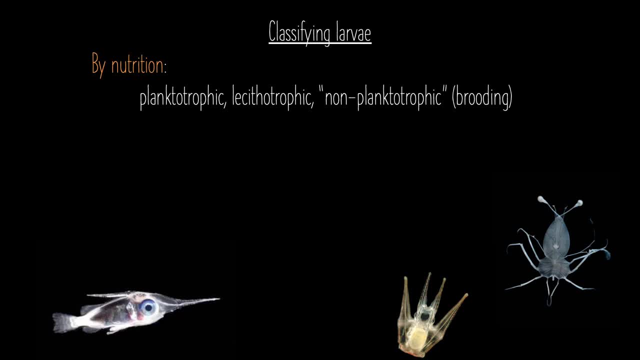 that refers to food or feeding, And so a larva that is planktotrophic is one that must feed in the plankton, The next term, lecithotrophic. The first part is lecitho, which refers to lecithin. 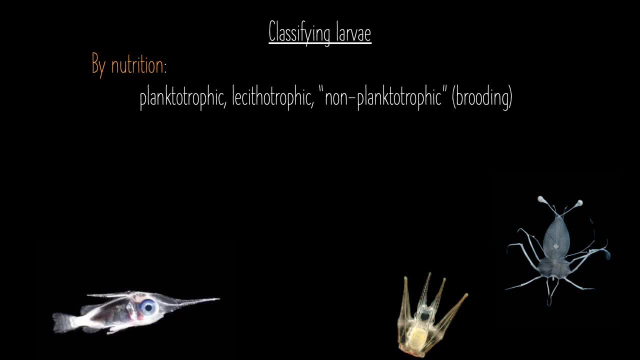 Lecithin or yolk, And then again trophic food or feeding. So a lecithotrophic larva is one that feeds on yolk, And what we mean by this is that this is an organism that gets all of its energetic requirements. 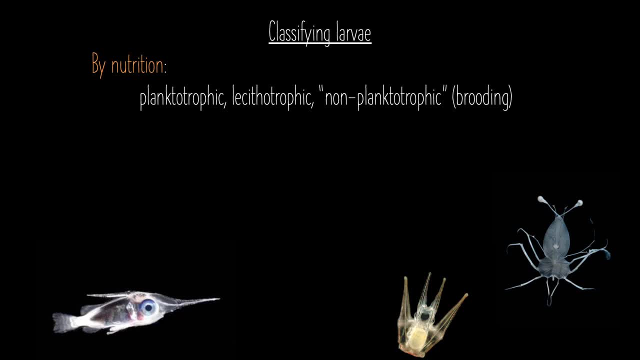 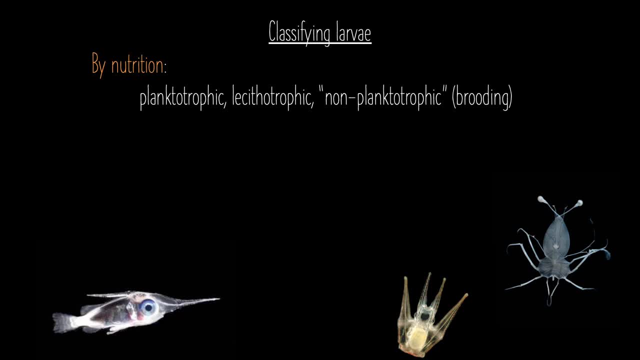 Lecithotrophic, Lecithotrophic, Lecithotrophic, Lecithotrophic, Lecithotrophic, or brooding, And what we're referring to here are those types of larvae that do not have to feed. 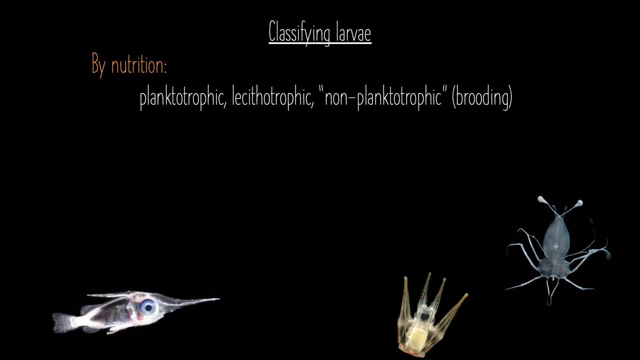 or at least not swim around pretending to feed in the plankton, like planktotrophic and lecithotrophic larvae do. But these are larvae that are brooded either on or within the body of the mother, or that may be retained within egg cases or egg masses. 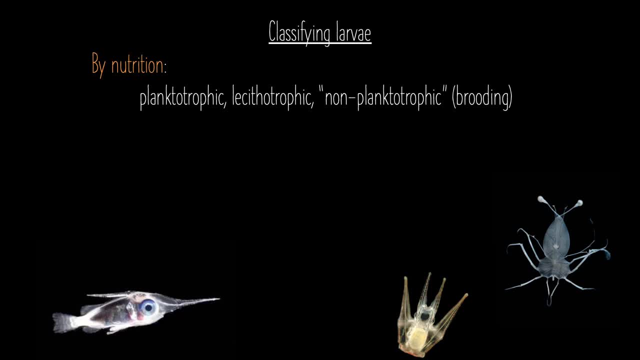 on the benthos, and so they're again. they're going to be getting their energetic needs from their mother and they're not going to have to feed in the plankton. we can also classify larvae by their habitat, and we have a series of terms here. 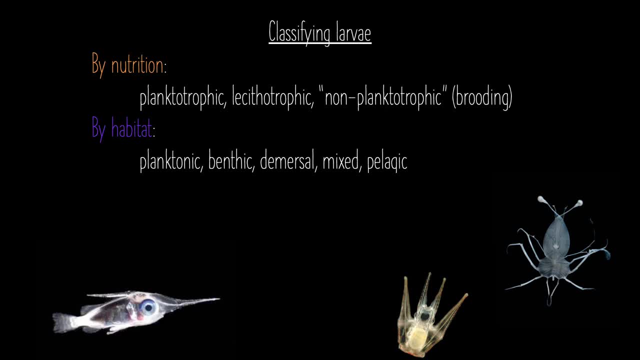 so: planktonic, meaning up in the water, column benthic, meaning on the bottom, on the benthos. demersal is a term that is used chiefly of fish and it refers to a fish that lives close to the floor of the sea or the ocean or a lake. okay, we don't really use that term with. 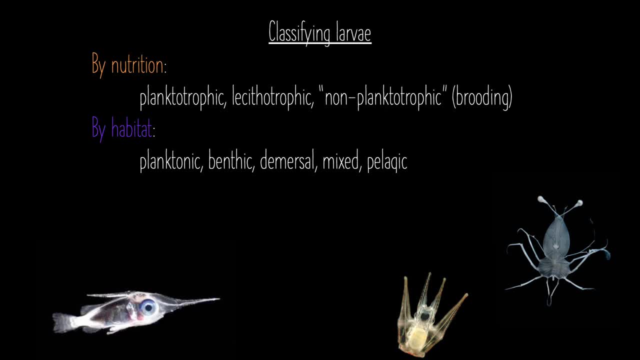 marine invertebrates, but it is a term that is used for fish and fish larvae. and then we have two other terms here: mixed and pelagic. pelagic refers to the open water and mixed refers to an organism that spends maybe part of its life cycle up in the water column and another part of its life cycle 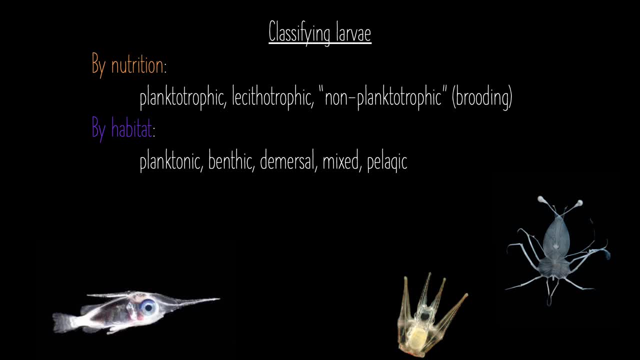 down on the benthos. i'll talk more about habitat use and how we can use those to think about larvae on the next slide, but i do want to present just a few more terms, and that is that there we can also classify larvae based on their parental protection. 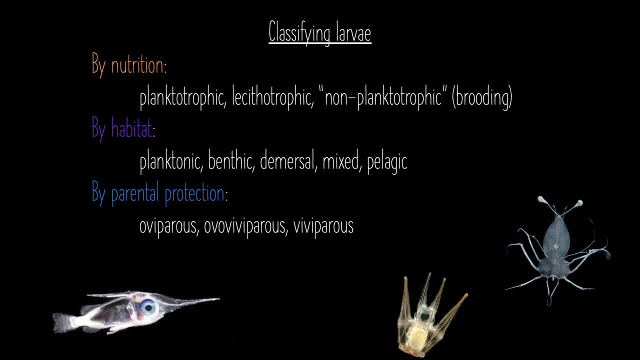 now, these terms- oviparous, ovoviviparous and viviparous- are terms that you may have seen before, if you've ever read anything about reptiles. oviparous is a situation in which an organism lays an egg and then the offspring hatch from that egg. that is. 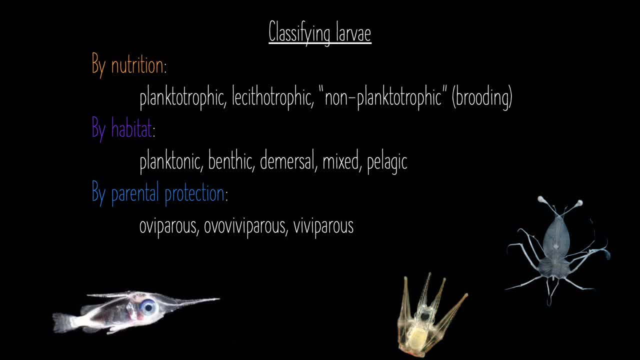 outside of the parent's body. ovoviviparous is a situation in which the offspring hatches from an egg retained within the body of the parent, And then viviparous refers to a situation in which an organism, a parent, births live organisms, and so there are no eggs involved in this situation. 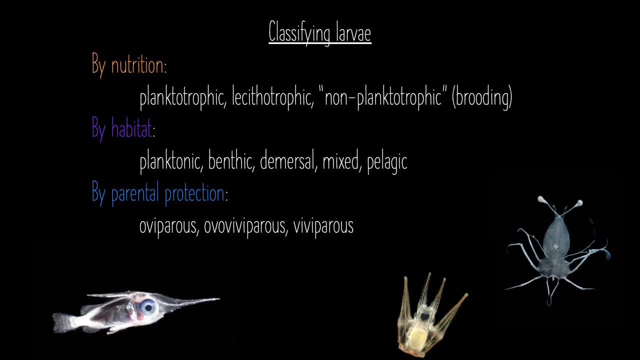 And again, these are terms that you might see if you're studying fish and fish larvae. certainly reptiles on land and those few reptiles that we find in association with the ocean, but they're not terms that we use commonly with marine invertebrates. 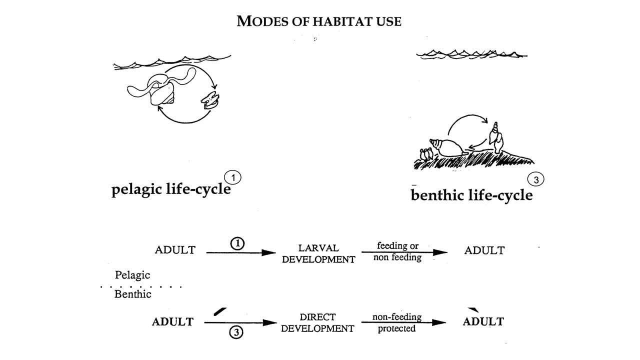 Let's go back and look at those terms that I mentioned on the last slide that I would clarify a little bit better. And this is a way of classifying larvae based on their habitat or their modes of habitat use. So one example: here on the left is depicted an organism that has a 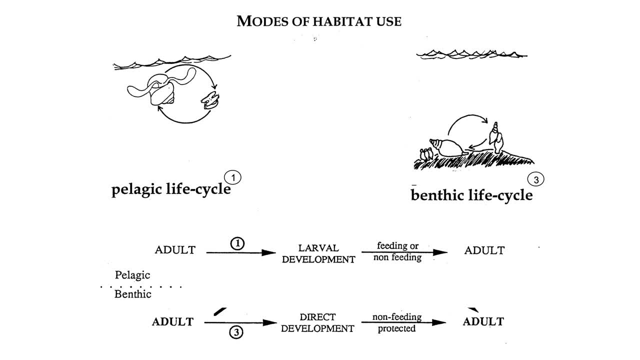 pelagic life cycle. In this case it's a pelagic life cycle that has a pelagic life cycle, that has some type of snail, that has a larval form, And for both life stages, both for the adult and the larva, their entire existence is found in open water. They never have any association with the 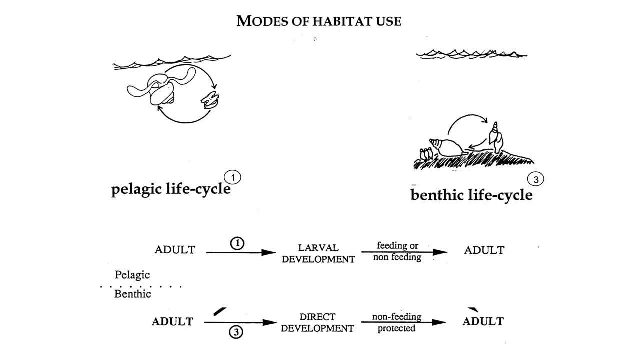 benthos, or with the bottom of the ocean. On the right side of the slide, we see an organism that has an entirely benthic life cycle. In this case, both the adult and the juveniles live their entire existence in association with the benthos, and they never go up into the water. 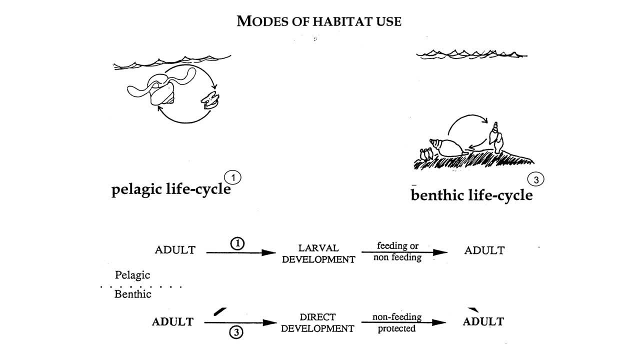 column. So an adult may deposit a set or series of eggs or egg masses or egg capsules on the bottom of the ocean and within those egg cases will develop little juveniles that ultimately will crawl away, hatch out and crawl away from the egg case and then grow up into an adult form. 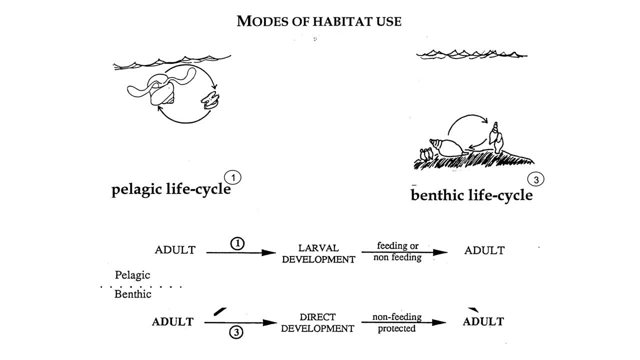 So for the- in the case of the first on the left, this is an example of an organism that has larval development. So there's an adult that will produce gametes that will turn into, you know, will fertilize and then develop into a larval stage. Ultimately there will be metamorphosis. and then that metamorphosis 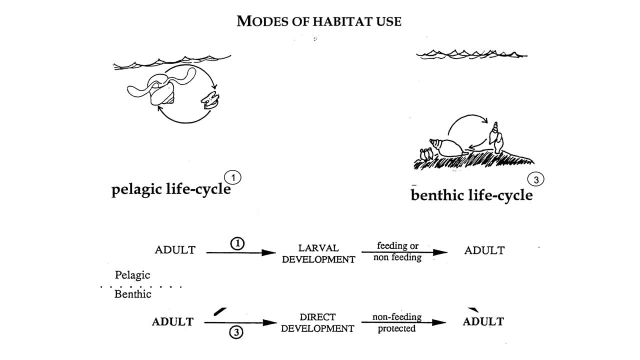 leads to a juvenile and then an adult stage. So in this case we have larval development. Sometimes this is called indirect development, because the the form of the organism changes between what the adult is and what it does- its function and morphology- and then what the larval form is and what it does in terms of its function and morphology. 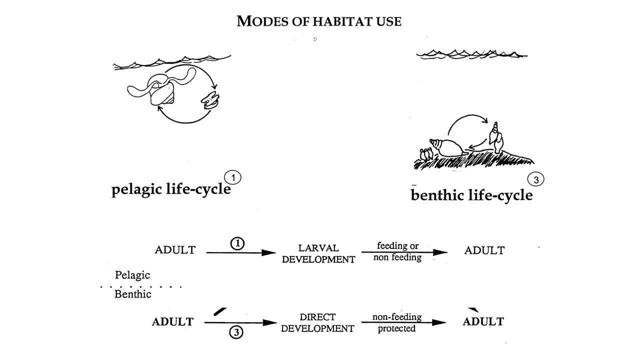 On the right is an organism that has direct development. The adult deposits eggs that grow directly into a juvenile that continues to grow once it leaves its egg case into the adult form. The third situation, as you might expect, the one here in the middle, is an example of an organism that has a mixed 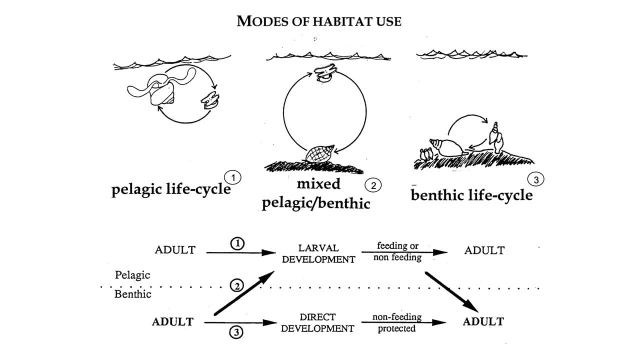 habitat use or, in this case, an organism that spends part of its life cycle on the benthos- in this case the adult- and alternates that with a stage of the life cycle that lives its existence up in the water column in the Pelagios. 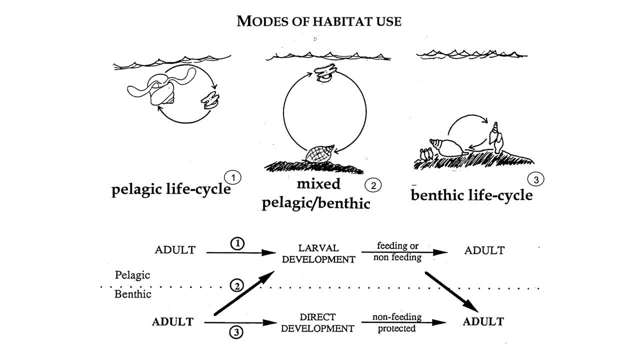 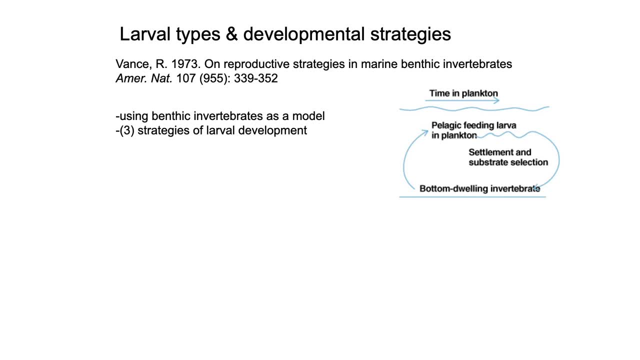 and this is an example. this is what we would call something that has a mix like mixed habitat use lifecycle. now I'd like to spend a few slides really kind of teasing out that situation- number two from the previous slide- where an organism has a mixed pelagic benthic type of habitat use lifecycle. what are? 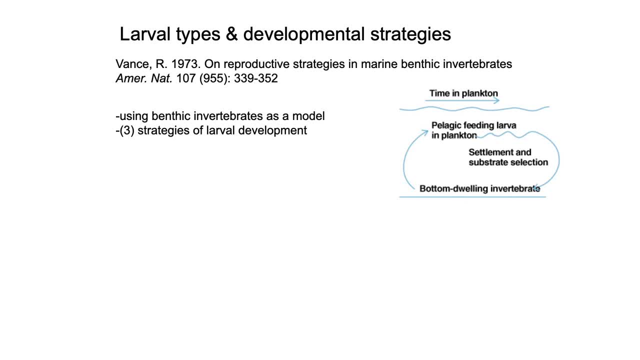 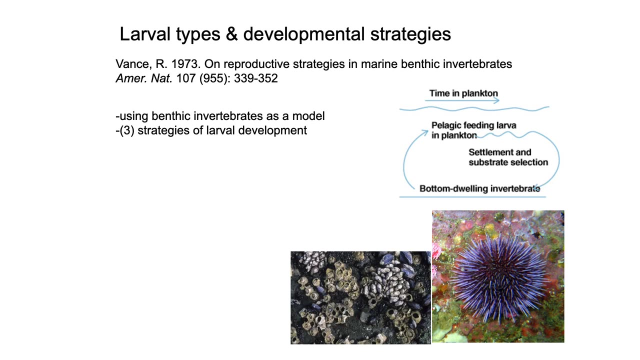 the different developmental strategies that mothers employ as they are producing their eggs and, ultimately, the offspring that will develop from those eggs. for many, marine invertebrates that have a bottom-dwelling adult, like the sea urchin or a barnacle, or corals, or marine sponges or marine worms. for many, 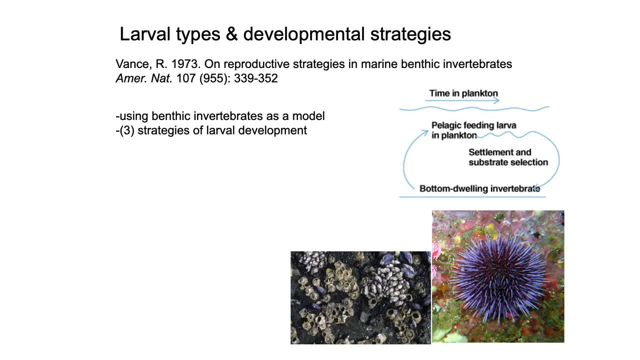 different types of marine invertebrates. one developmental strategy is to produce larvae that have to feed in the plankton, and you can see that there are a number of different types of invertebrates that have to feed in the plankton and, again based on the nutrition, these are going. 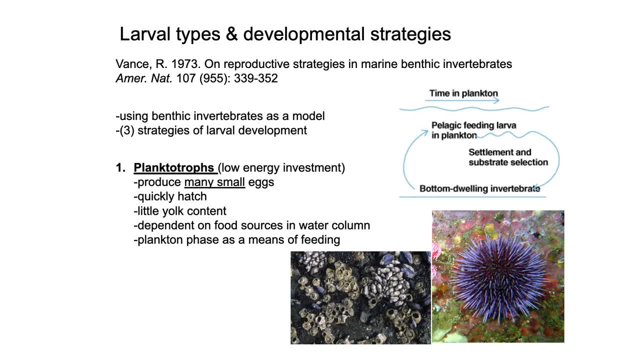 to be organisms that we refer to as planktotropes. so specifically, the larvae are planktotrophic larvae. that means that they have to feed in the plankton, and for these organisms mothers will produce many small eggs, and each individual egg has a very low yolk content, which means not much in the way. 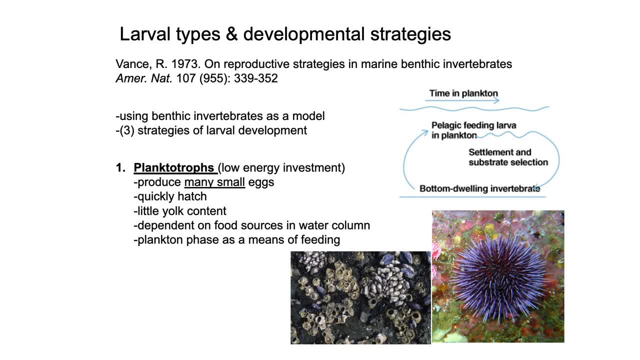 proteins, lipids and carbohydrates. And if you convert those biochemical constituents into energy, there's for an individual egg a very low energy investment on behalf of the mother. So because there's not a lot of energy in the individual egg, the larva that develops from that 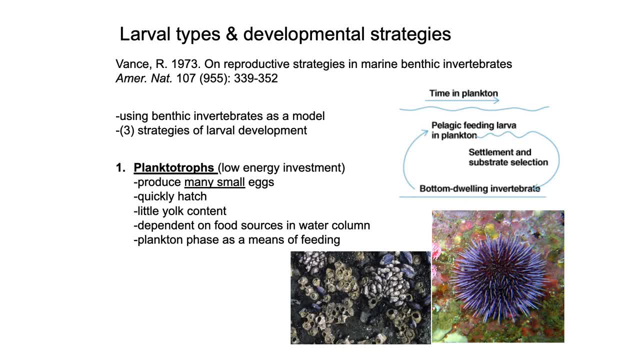 egg has to feed in the plankton, And the planktonic phase then serves primarily as a means of feeding. So these are the kind of classic little feeding machines that I was speaking about earlier in the beginning of this lecture. Another strategy that has evolved for organisms. 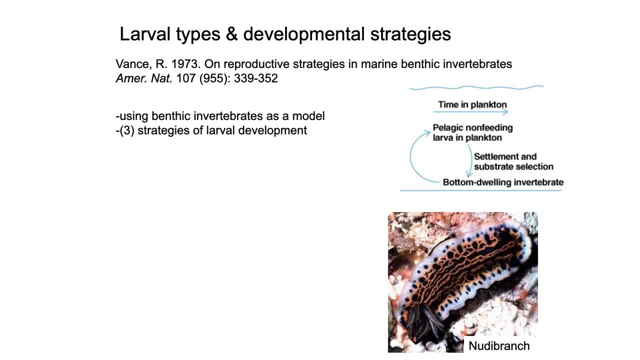 that have bottom-dwelling adults, like this nudibranch or perhaps a marine snail. some corals are similar to what I'm about to describe, and that is for these organisms with bottom-dwelling adults that also produce a lot of energy. So these are the kinds of organisms that have bottom-dwelling. 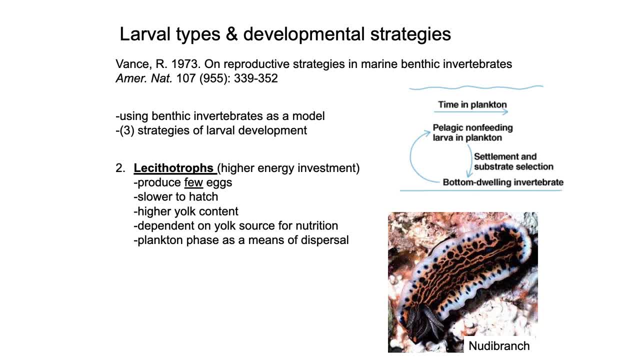 adults that also produce a lot of energy. So these are the kinds of organisms that have bottom-dwelling adults that also produce a lot of energy. So these are the kinds of organisms that have bottom-dwelling stage, In this case, if the larvae develop from very large eggs that have a high yolk content. 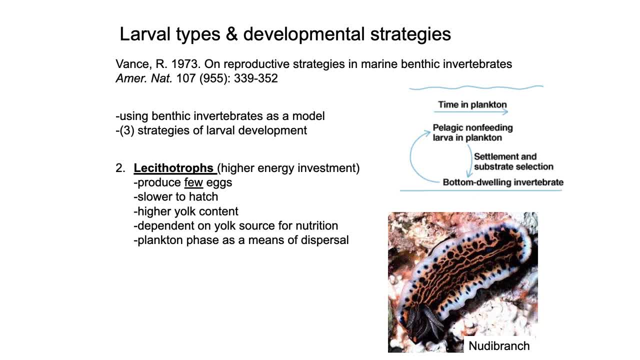 so plenty of proteins and lipids and carbohydrates. very high energy. investment, then, on behalf of the mother, in any individual eggs. that mother will therefore then only produce a few eggs. The larvae may be slower to hatch out of those eggs, but they are entirely dependent on that. yolk source for nutrition. So if the larvae develop from very large eggs that have a high yolk content, so plenty of proteins and lipids and carbohydrates, very high energy investment then, on behalf of the mother in any individual eggs. so plenty of proteins and lipids and carbohydrates. very high energy investment then, on behalf of the mother in any individual eggs. 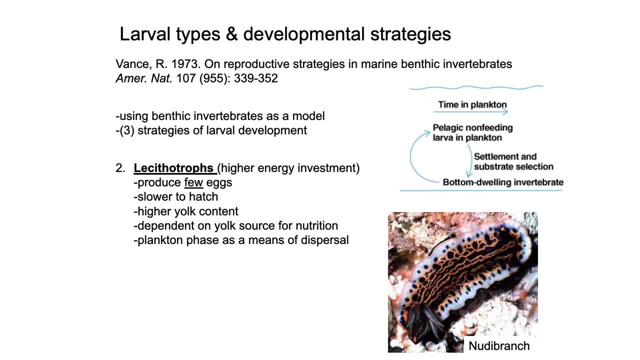 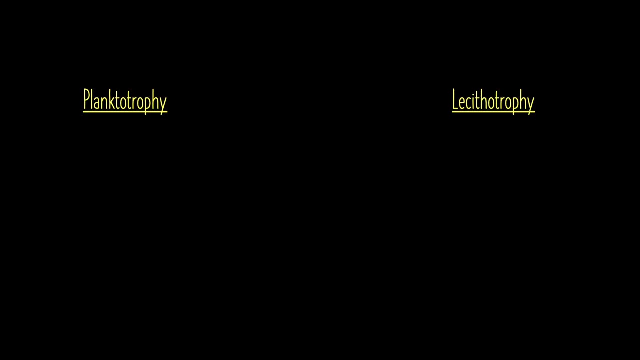 and therefore their time spent up in the water is used solely as a means of dispersing away from where the mother is located. These are lesothetrophs and they have evolved a lesothetrophic developmental strategy. These two developmental strategies, you can think of them as existing on two ends. 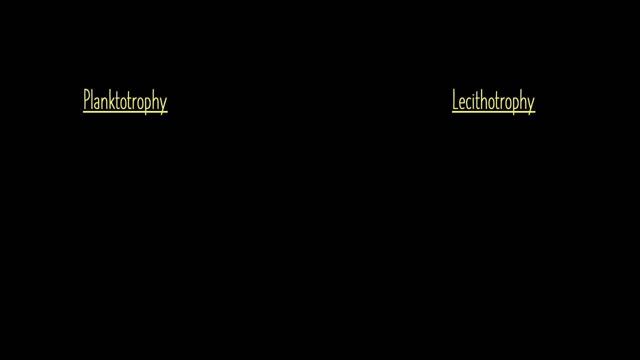 of a spectrum. On the one side we have planktotrophy, so feeding in the plankton, and on the other we have lesothetrophy, feeding off of energetic reserves in the yolk. And associated with those two developmental strategies are a suite of different. 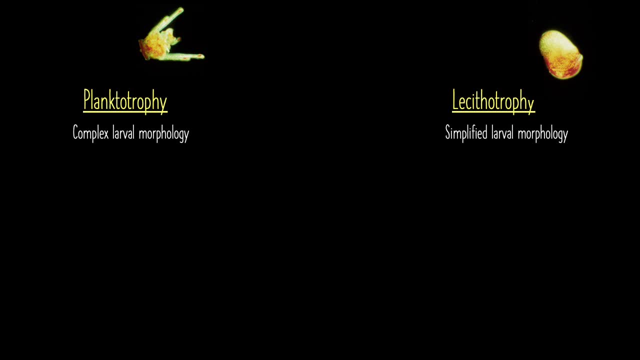 characters that correlate with those different strategies. So, in the case of a planktotrophic larva, the larva will have a very complex, plain morphology because it has a series of different feeding structures that have to be extended away from the body in order to capture phytoplankton. 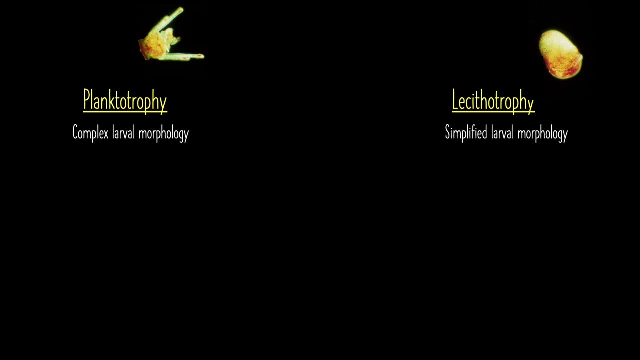 whereas in the case of the lesothetrophs, those larvae will have a very simplified type of larval morphology And they will have lost, evolutionarily speaking, any feeding mechanisms that they might have had in previous times. The mothers of the plankton. 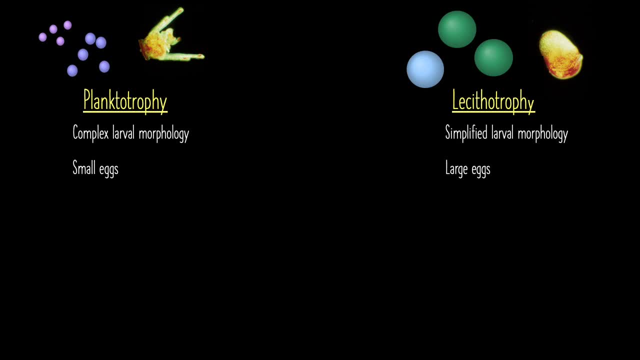 Planktotrophs will produce many small eggs, whereas the larvae of the lecithotrophs will produce only a few large eggs and thus, in terms of fecundity, which refers to how many offspring an organism produces, the planktotroph has very high fecundity, whereas the lecithotroph. 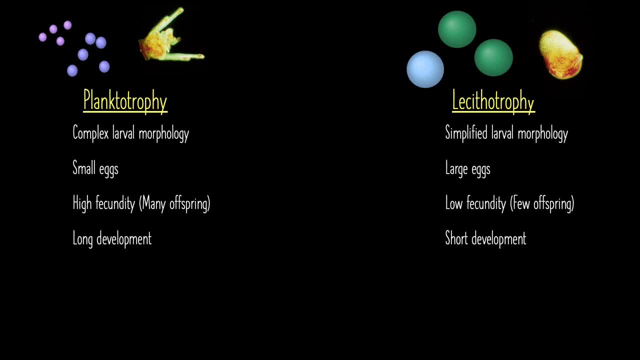 has very low fecundity Because a planktotrophic larva has to feed in the plankton, it may have a very long developmental period, whereas the lecithotroph because it already has all of the energy that it needs to develop to metamorphosis in the egg that it's developing. 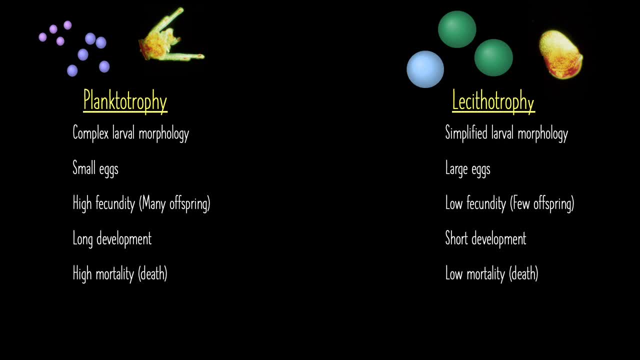 from then it may have a very short development. The planktotroph may experience high mortality because it is spending a longer time swimming around in the plankton trying to collect food, so there's more time available for predators to find it and to eat it, whereas for the lecithotroph it may have much lower mortality. 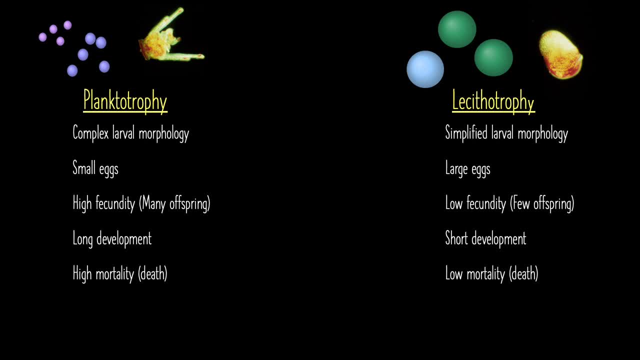 And then again, in the case of mortality, we're referring to death. And then the last character here is that for the planktotroph, these organisms may have very high dyspepsia, They may have very low dispersal due to the fact that they're spending a very long period. 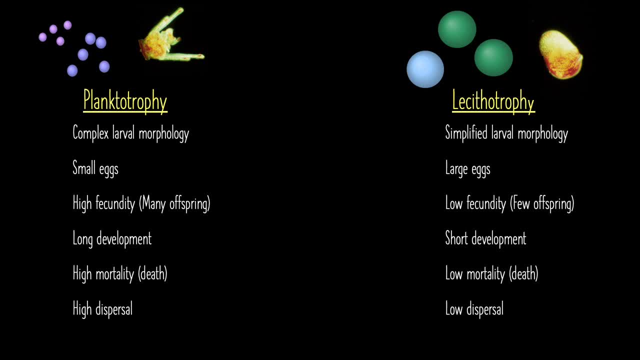 of time in the plankton, and thus they can be taken far away from where the mother originally spawned them into the water. whereas for the lecithotroph they may have very low dispersal in comparison to what the planktotrophic larva has. 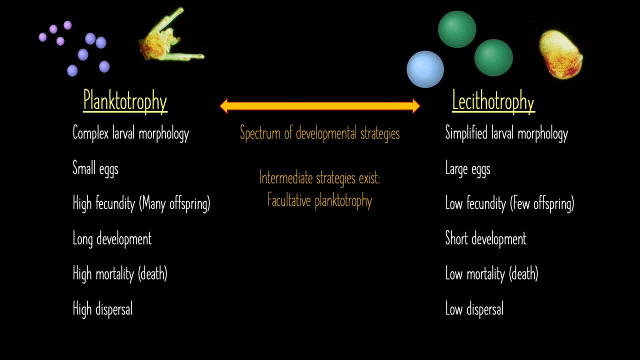 So again, this is a. these two developmental strategies exist along a spectrum of different types of developmental strategies, and intermediate strategies actually exist, So there's something called facultative planktotrophy, and these are organisms that have all of the feeding structures that are necessary for collecting food from the plankton, and yet 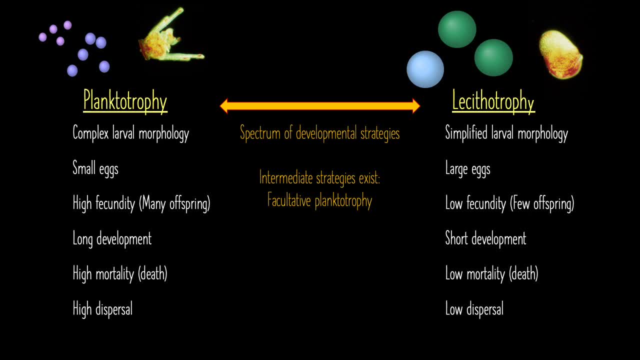 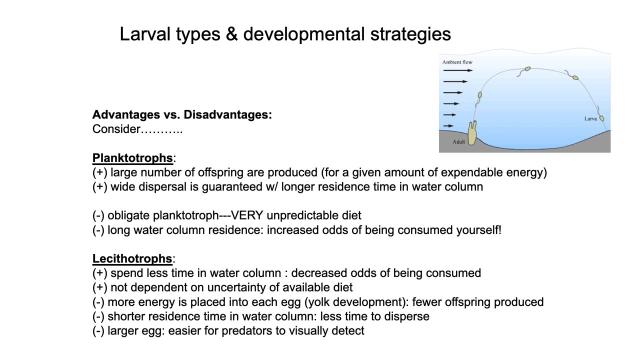 they develop from eggs that are large enough that they do not have to feed. So that's a type of intermediate strategy that falls within the spectrum of planktotrophy to lecithotroph. What are some of the advantages and disadvantages to these two different strategies? 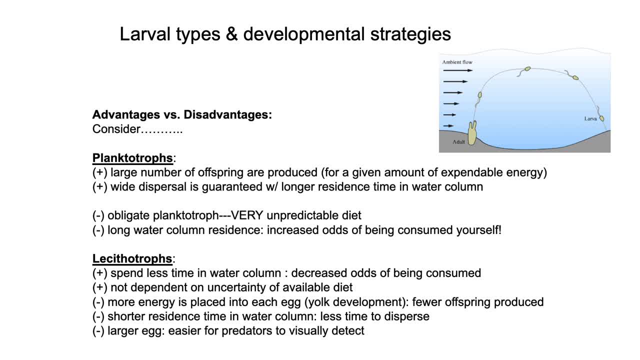 Planktotrophs. you know, an individual mother will produce a large number of offspring for a given amount of energy. So let's say that if she's going to put 100 units of energy into development and any individual egg is going to only have one unit of energy, then she can make 100 offspring. 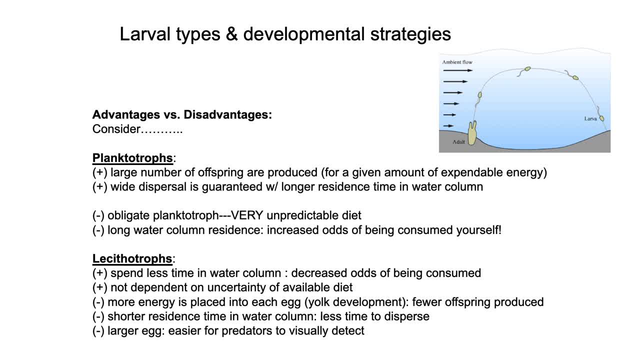 for a given about 10 weeks where they don't need to keep those eight, no matter how they breed. If she doesn't need to keep them, there's an additional 60 units of energy to allow them to form enough for her offspring to be able to fertilize and to look bottomless. 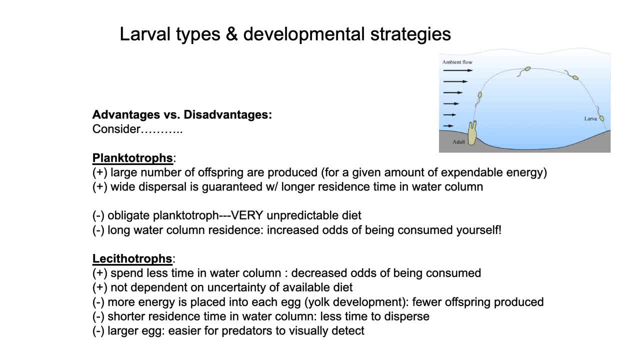 in mid- nurturing to make her offspring more unfe. Audience question Why dispersal is probably guaranteed for these organisms? because they're going to have a very long residence time in the water column, Meaning the longer that the larva is out there, the more likely it is going to be dispersed. 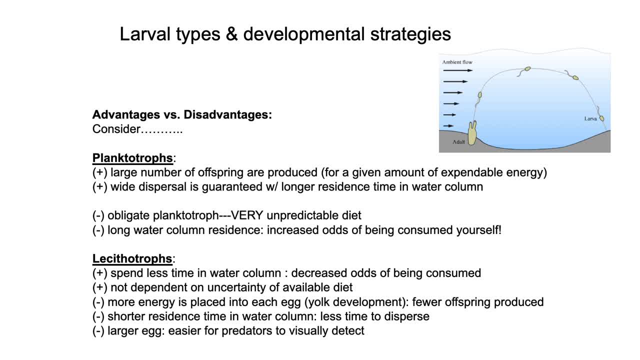 far and wide from where the adults are located, develop. that's very different from the facultative planktotroph that i mentioned on the previous slide. an obligate planktotroph has a very unpredictable diet. it could be that you, as an individual larva, hatch out and there's phytoplankton everywhere where you happen to. 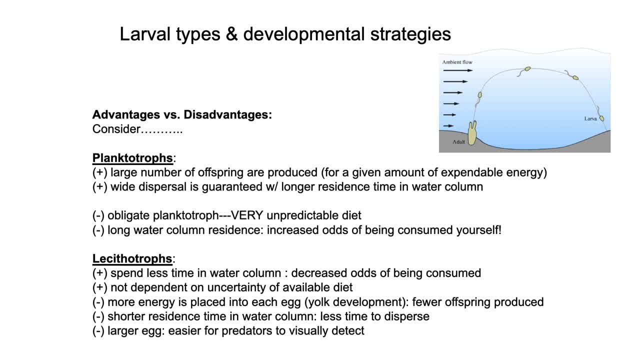 to hatch out, and so you're in this food buffet and you're living the lush life. that's great for you. but it could also be a situation where you hatch out and you find yourself in an area where there's very, very low levels of phytoplankton food, and that is not a good thing for you at all. 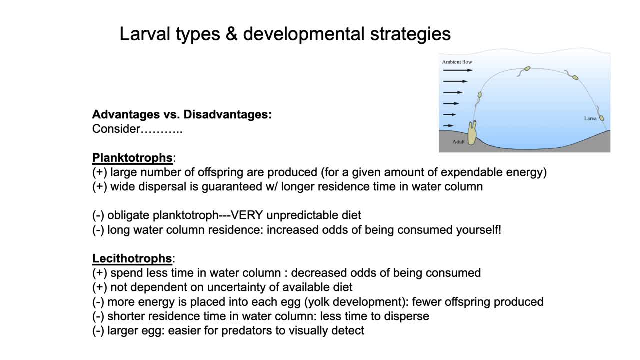 as an obligate plankton trove. another disadvantage is that the longer time that you spend swimming around in the water column, the more likely it is that you're going to be consumed yourself, meaning more likely that you're going to be eaten by something else. for the less of the trove these organisms. one of the advantages is that they spend less time. 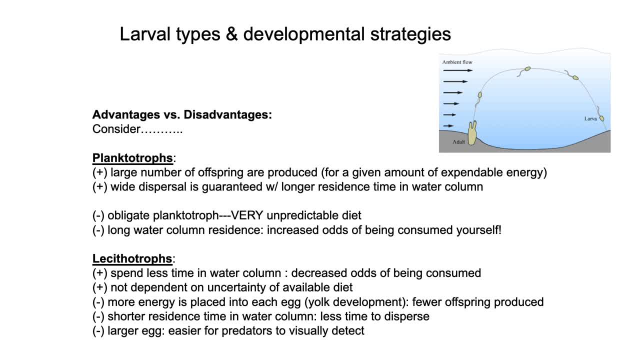 in the water column, and therefore your odds of being eaten by something else are much lower. Another advantage is that you're not dependent on the uncertainty of any available diet, because you have all of the energy that you need within the egg that you're developing. from A disadvantage, though, 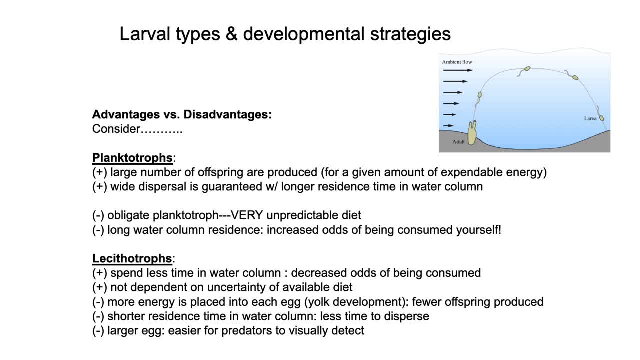 is that because a mother is putting more energy into an individual egg, then that means she's able to only produce fewer offspring. So again, if we go back to this idea of: let's assume a mother has 100 units of energy that she can put into her development and she puts 10 units into. 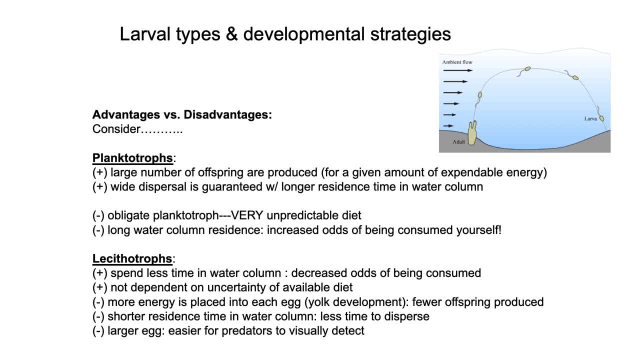 an individual egg, then she's only able to make 10 offspring, whereas the plankton trope was able to make 100 offspring. Another disadvantage for the less of the tropes is that because they spend less time on the egg, they're able to produce less of the energy that they need. So if you're 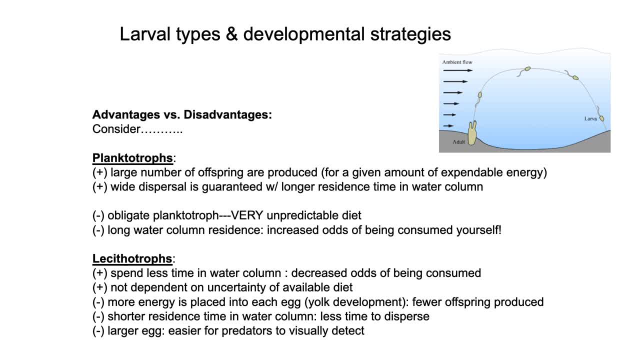 in the water column they will not disperse as far as a plankton trophic larva will. And another disadvantage is that a larger egg is easier for predators to detect visually. It's this old idea of a larger egg. here is kind of a larger target for a predator to see and to find. 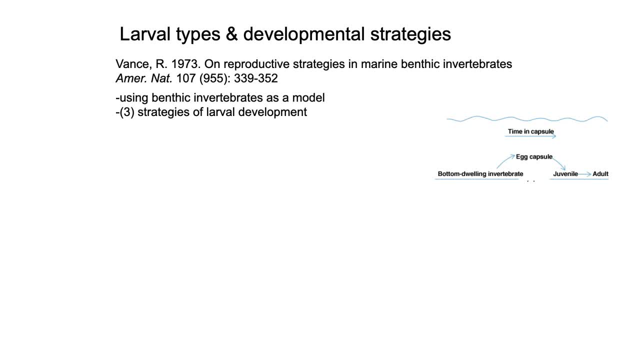 The third type of developmental strategy is the ability to detect and to find. The third type of developmental strategy that was identified by Vance is a situation in which you have a bottom dwelling invertebrate, perhaps something like this blue-ringed octopus or many other cephalopods, octopus primarily, also marine snails, some marine snails, But it's a situation. 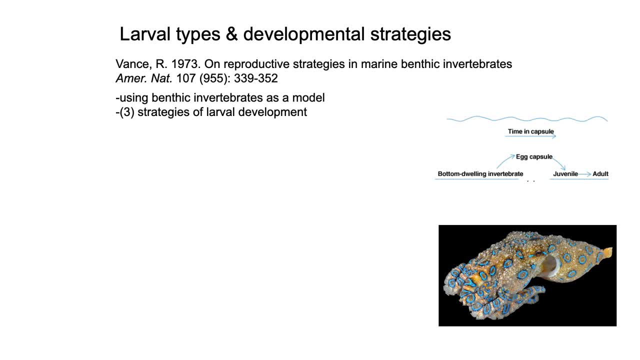 in which you have a bottom dwelling invertebrate that deposits eggs within an egg capsule that is attached to the benthos and within the bottom dwelling invertebrate. you have a bottom dwelling invertebrate that is attached to the benthos and within that egg capsule, a larval stage, if there is one. 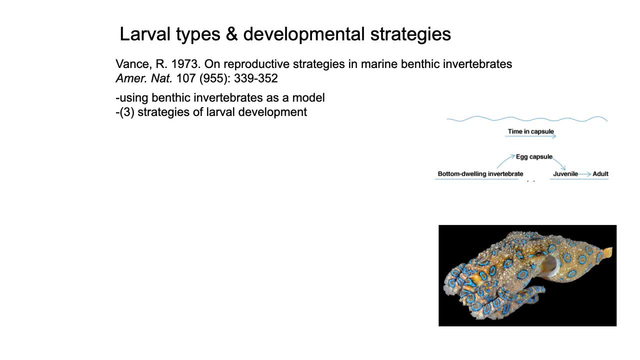 develops, or the organism may develop directly into a juvenile stage. Eventually, the juvenile is what hatches out of the egg capsule and then crawls away or swims away as an adult. And this is a situation in which you have non-pelagic or direct development And it's kind of like less of the 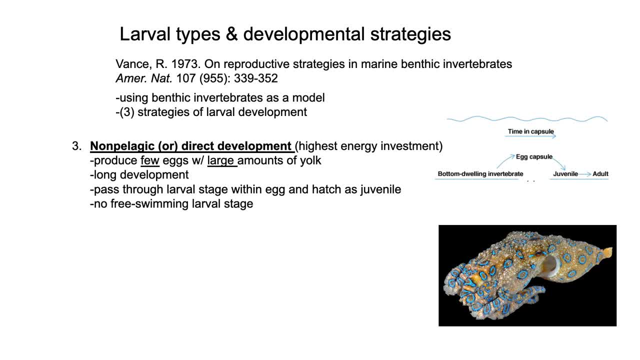 trophy, taken to the extreme. So mothers will produce only a few eggs in the egg capsule, and each individual egg has a very large amount of yolk. The larvae or the juveniles undergo long development. They might pass through a larval stage, but that larval stage stays retained within. 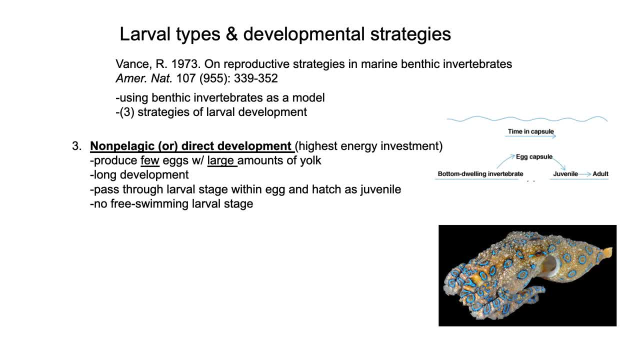 the egg in the egg capsule And then ultimately there is a hatching as a juvenile And again there's no free swimming larval stage for these organisms. An advantage of this type of development is that it reduces the number of eggs that are hatching. So if you have a larval stage and you 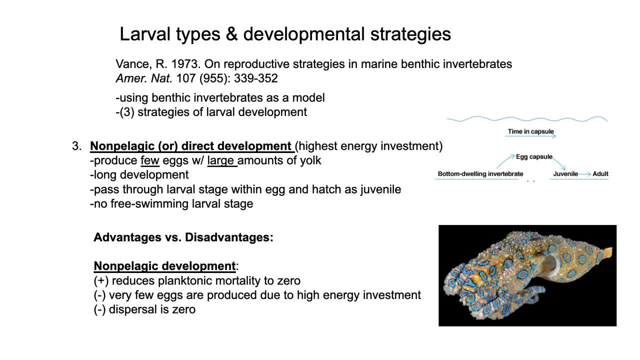 have an egg capsule and you have an egg in the egg capsule. it reduces the number of eggs that are hatching. It reduces planktonic mortality to nothing, to zero, because there is never a situation in which the organism is up in the plankton. A disadvantage, though, is that any individual 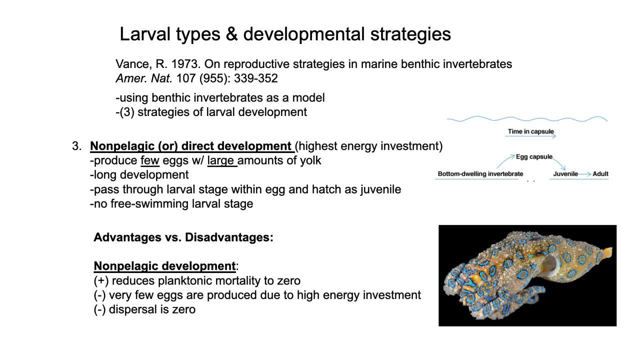 mother only produces a few eggs because each egg has such high energetic investment. And another disadvantage is that the dispersal is effectively zero. So because of the juvenile hatches out right from where the mother attached the egg capsule to the egg capsule. So if you have a 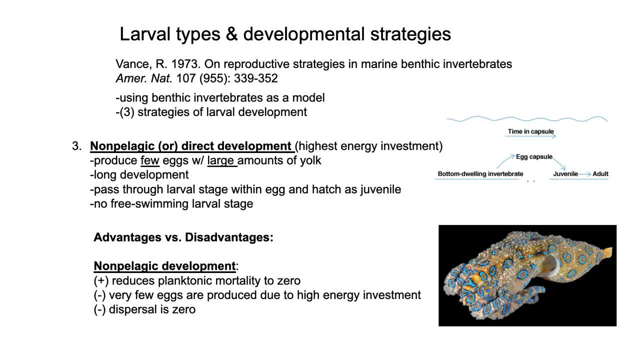 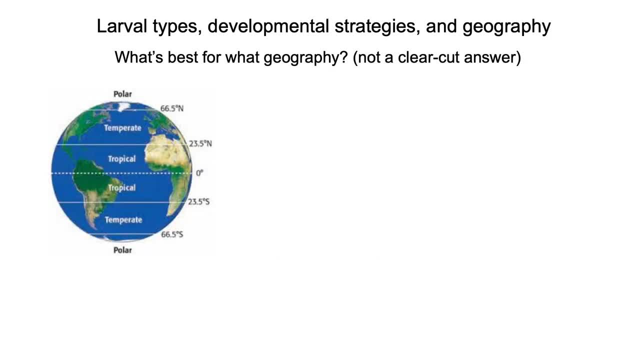 single egg capsule to the benthos, then the. there is no dispersal at all during the, the larval or the developmental period. What can we say about the prevalence of certain larval types or specific developmental strategies and particular geographical regions, Or in other words, what's best for what? 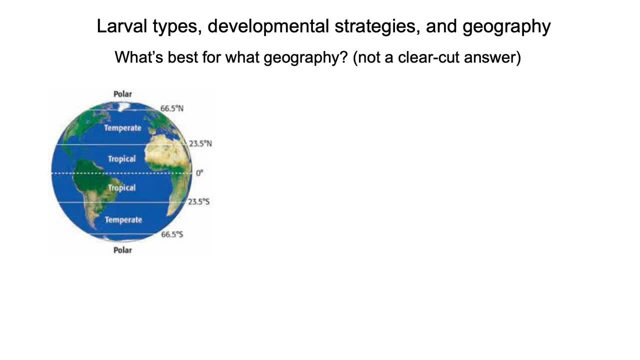 geography. The short answer is that there's really not a clear-cut answer, but there are some broad examples. The first is that in polar waters, non-pelagic development is more common. This has to do with the fact that there's really only a narrow window of time during the summer when there 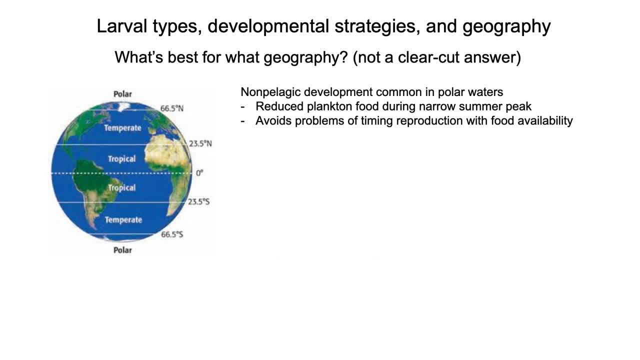 is significant phytoplankton food availability for developing larvae in the water column. That narrow window of time coincides with when there is significant light due to the increase in solar light radiation as the the region progresses from spring into summer, and when warming waters fuel the formation of a phytoplankton bloom. 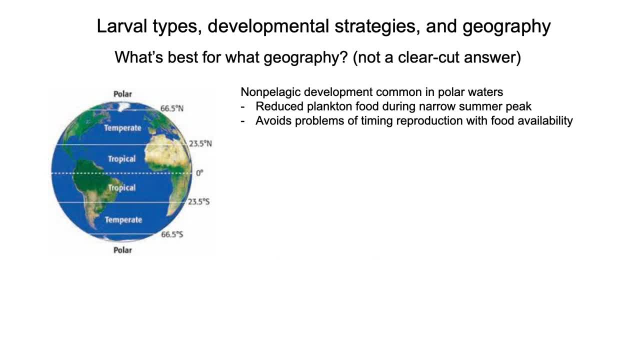 So if you're an adult and you are trying to time your reproduction with the availability of food for your larvae, it may be a better strategy to have evolved a non-pelagic form of development In temperate and tropical waters, where the predictability of phytoplankton food for your larvae is. 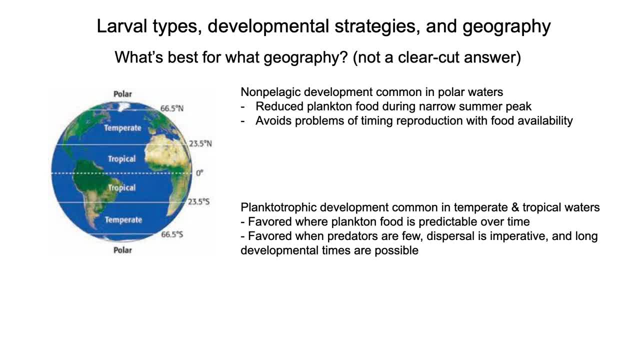 higher, even in the tropics, where the amount, the overall amount, of phytoplankton food is really low, at least it's still predictable you're more likely to find planktotrophic development. You may also find that planktotrophic development is favored in those areas where there are few predators. 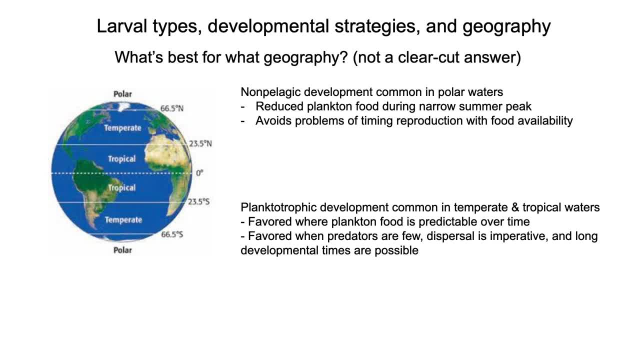 where maybe it's imperative for there to be dispersal, and also in those areas where it's possible to have long developmental times In the situation of less lithotrophic development. less lithotrophic development will be found in areas where, compared to non-pelagic development, 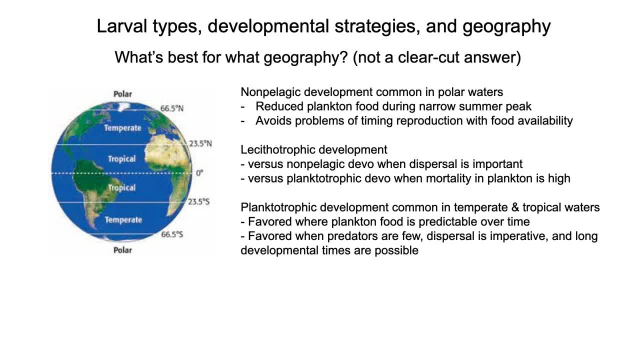 dispersal is important, And also when you're comparing less lithotrophic development to planktotrophic development, less lithotrophic development will be favored in those areas where planktonic mortality is high, And so it would be more important for larvae to get out. 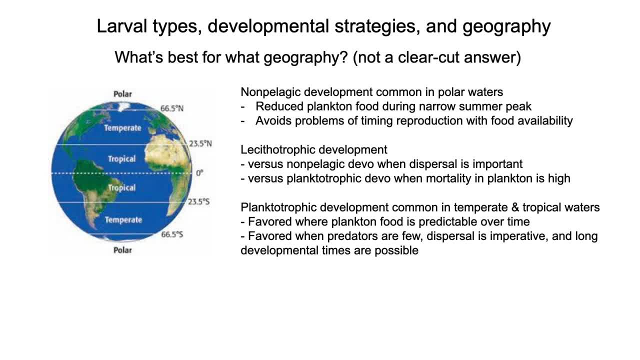 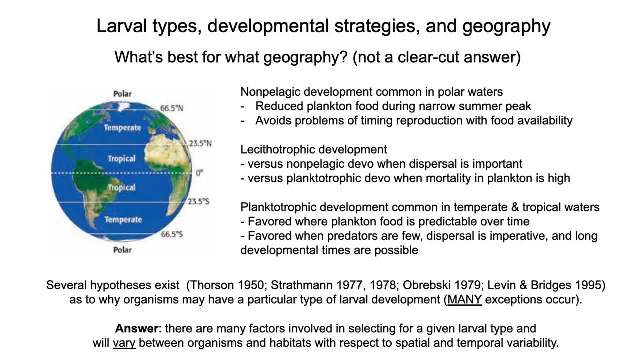 of the water column and metamorphose into the juvenile stage more quickly. Several hypotheses exist as to why organisms may have a particular type of larval development. There's been some fascinating research done over many decades in terms of these types of questions, and I encourage you to at least start with some of 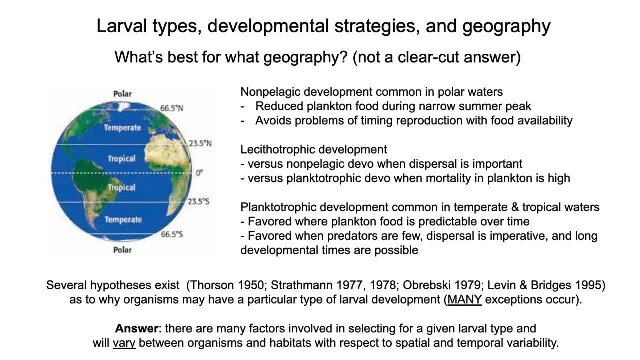 the references that I've listed here, But note that many exceptions occur. So, while the short answer was that there was not a clear-cut answer in terms of what's best for what- geography- the longer answer is really that there are many factors involved in selecting for. 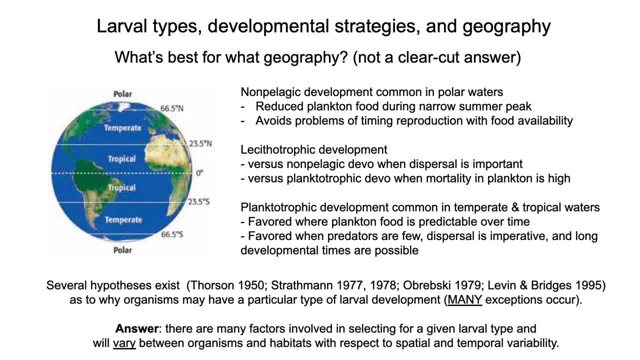 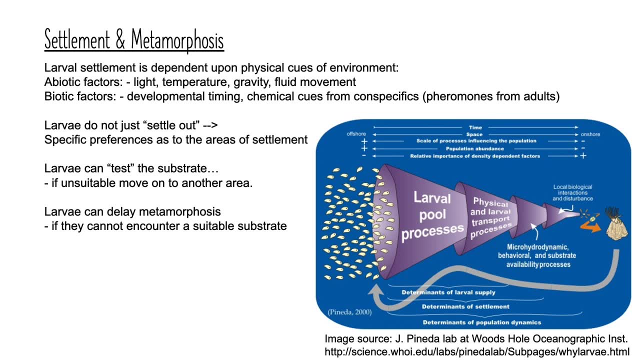 a given larval type, And these factors will vary between organisms and habitats, both in space and in time. Ultimately, larvae will reach a point in which they will undergo metamorphosis and ultimately settle into the benthos, into either the juvenile or the adult habitat. 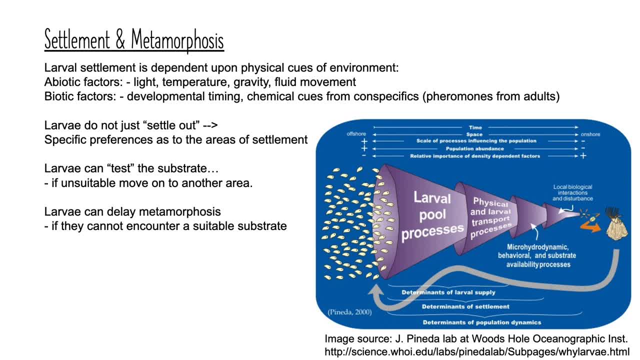 And settlement is dependent on a number of different physical cues. Those cues can include abiotic factors such as the amount of light or the temperature. It could be gravity or the movement of fluid water flowing over a particular substrate. The settlement may also be dependent upon 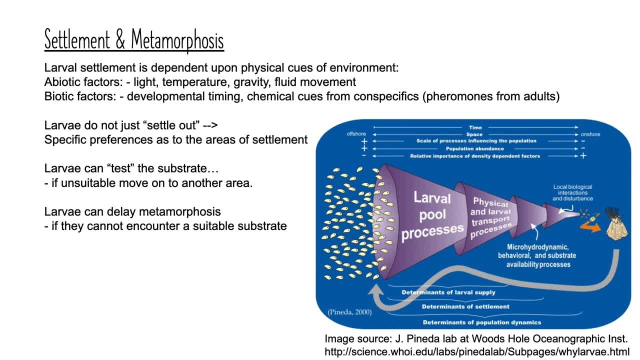 biotic factors as cues, such as just developmental timing, or chemical cues from conspecifics, and that means other organisms that are of the same species. In particular, it may include pheromones that are being released from adults that tell larvae that this is a good place to settle. I should emphasize that larvae do not just quote, unquote, settle out. 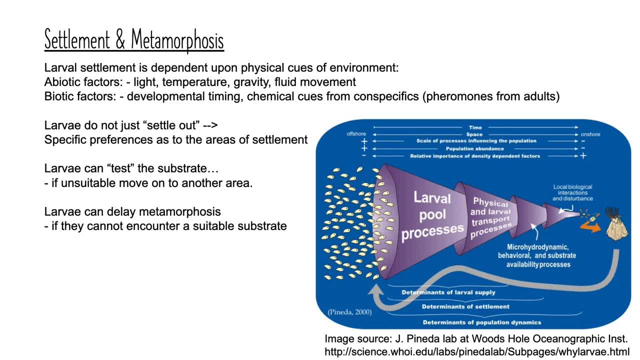 There are specific preferences exhibited by an individual larva for a particular area of settlement, And a larva- or larvae plural- can test the substrate, So they may chemically taste it, They may assess whether or not the water flow is appropriate or whether or not it has the right light availability or the right temperature, etc. 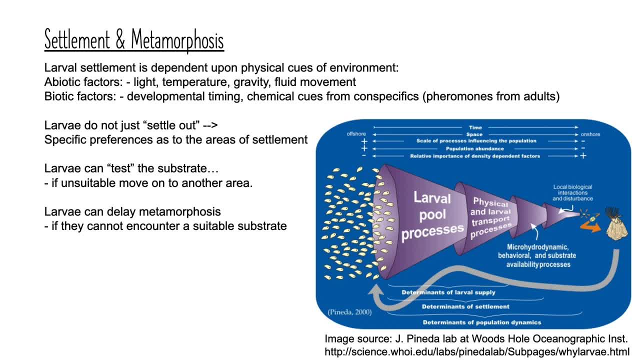 Any of those cues that I just mentioned, And if an area is unsuitable, then a larva can move on to another area and test that area. I should also also mention that larvae can delay metamorphosis if they cannot encounter a suitable substrate. 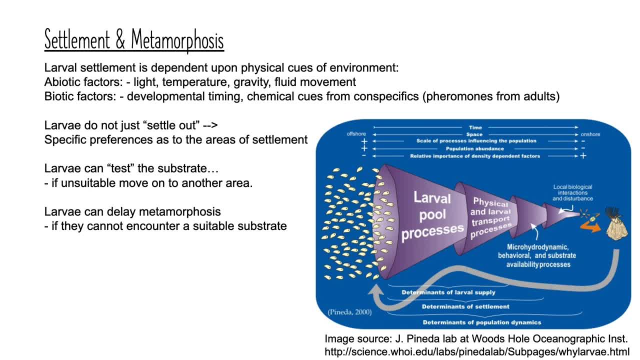 I should also mention that larvae can delay metamorphosis if they cannot encounter a suitable substrate, and some larvae have jump states to help them, but it's not healthy for them to test it. larvae have the capability of shutting down their metabolic processes to an exceedingly low level. 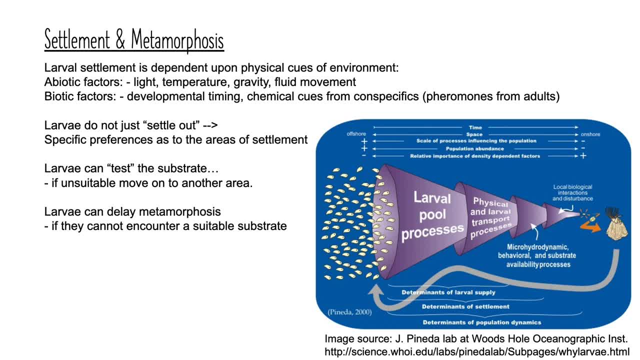 until such time that that they do encounter an area that is appropriate for settlement. if you're interested in understanding more about settlement and larvae, then i encourage you to visit the website of jesus panetta at the woods whole oceanographic institute, which is where i sourced this particular image that highlights the different 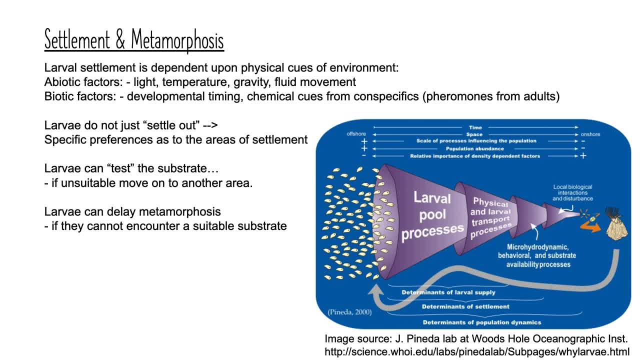 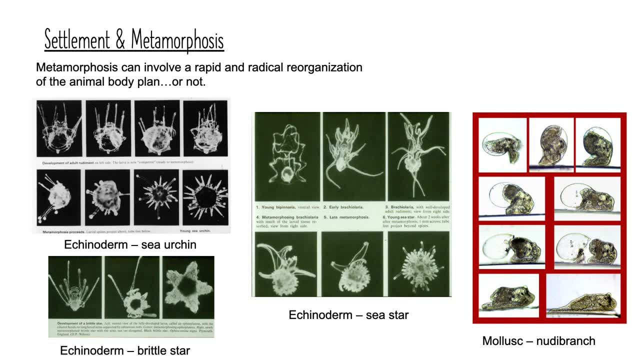 biotic and abiotic factors that affect settlement. in many marine organisms, settlement and metamorphosis are often coincident, meaning they happen at this around the same time, and metamorphosis can involve a very rapid and radical reorganization of the animal body plan, similar to what we saw in the last video. 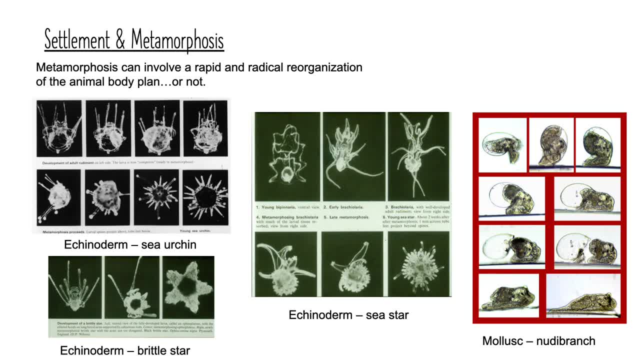 see with many of these different echinoderms that I've depicted for you here. In the case of the sea urchin, the pluteus larval form will metamorphose into the juvenile by resorbing the larval arms that stick out away from the body and shunting the energy that comes from the breakdown of those. 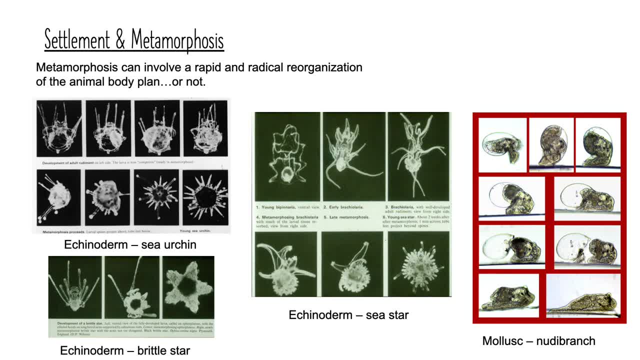 larval structures into the formation of juvenile structures. The brittle star also has a pluteus larval form that undergoes this very radical reorganization into the juvenile. that is star shaped, And a sea star will turn a bipenaria or brachylaria larva into a juvenile sea star. 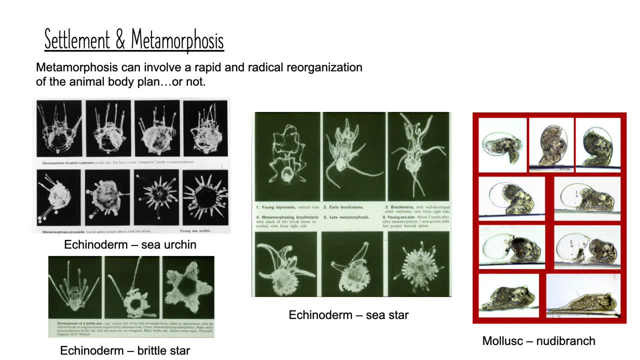 also with a very rapid and radical reorganization. Or it could be that metamorphosis is not very rapid or radical And we see something like that here with the nudibranch, this mollusk as it tests a substrate for settlement and then slowly kind of crawls away from the larval shell and becomes a juvenile. 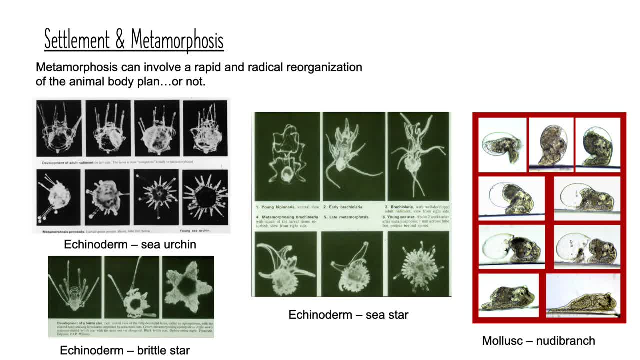 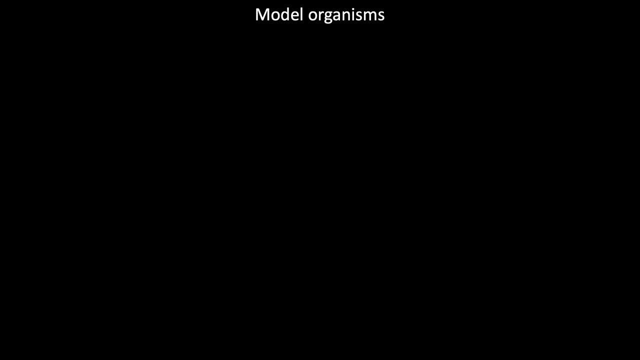 The metamorphic process is not very radical. It's not this kind of exceedingly large transformation from something that's very different to something in the larval form to something that's very kind of different in the adult form or the juvenile form. Before we finish up, I want to put larvae and the life cycles of marine invertebrates. 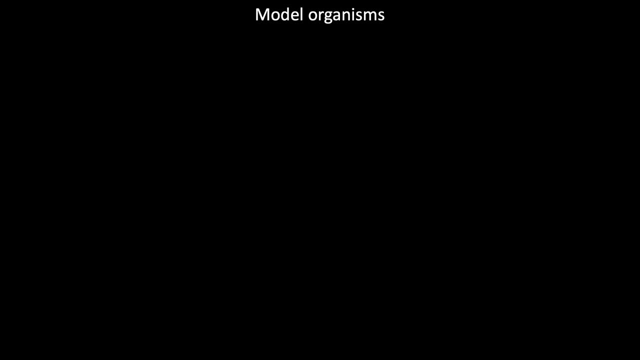 in the context of modern biology. Many biologists and students of biology understand that model organisms, so organisms such as C elegans or Drosophila or zebrafish, the laboratory mouse or Arabidopsis. these organisms are exceedingly important if what your goal to do is to experimentally 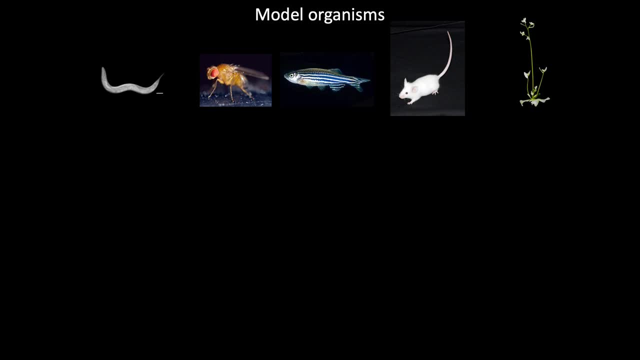 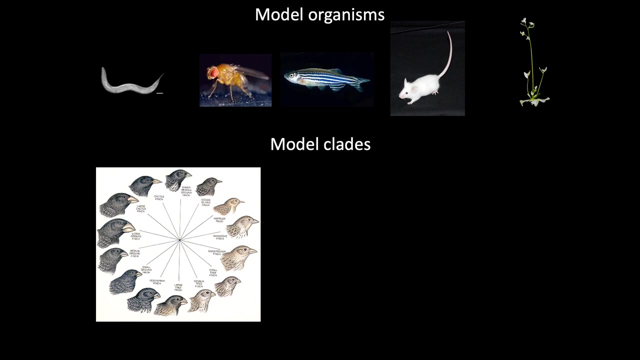 investigate biological processes to great depth. These types of organisms facilitate the precise dissection of causal relationships in biology. If you're more interested in evolutionary questions, then those types of biologists will employ what are known as model clades, or groups of organisms that are closely related to one another, in which there are 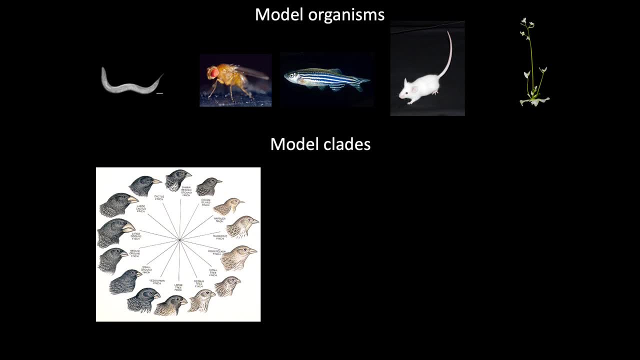 characteristics that differ between representative members and allow for evolutionary questions about the origin of traits. One of the classic model clades are the finches of the Galapagos, or Darwin's finches, And these are a group of species that are closely related and yet have evolved significant. 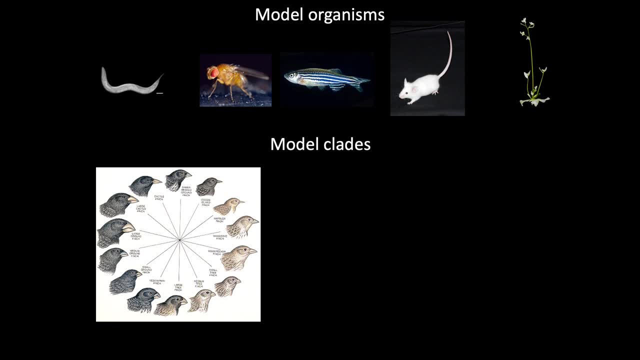 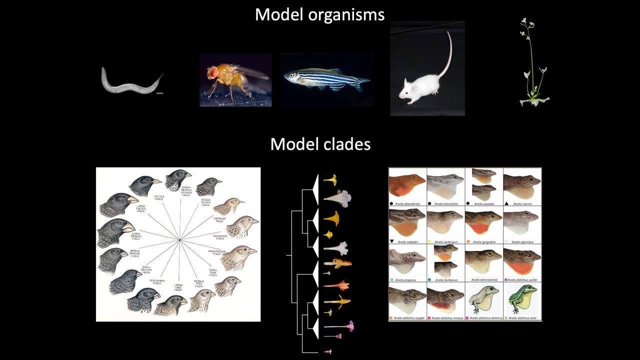 differences in the function and morphology of their beaks, And other examples of model clades include the Enolus lizards that have been studied by Jonathan Losos and his colleagues and students, and also a group of flowers that are known as Mimulus. That's the genus. 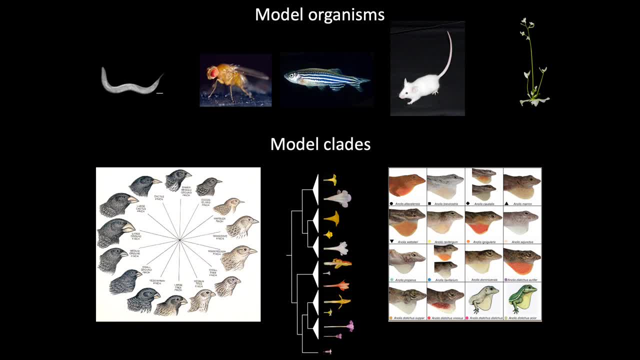 They're commonly called monkey flower Model clades. in model clades the phylogenetic relationships are very well established, and studying model clades allows for detailed morphological and behavioral knowledge about different species, so they also have a very important place in modern biology. 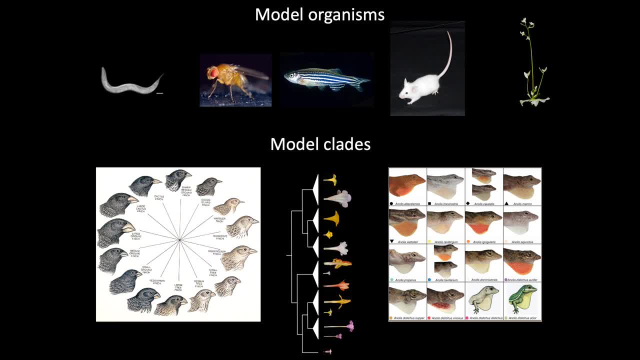 Where do larvae and life cycles of marine invertebrates fit in in modern biology? Well, they actually fit in in the phylogenetic relationships that we have is a process called epigenetic. The phylogenetic relationship of the phylogenetic relationship between pod and cell is a process called epigenetics. 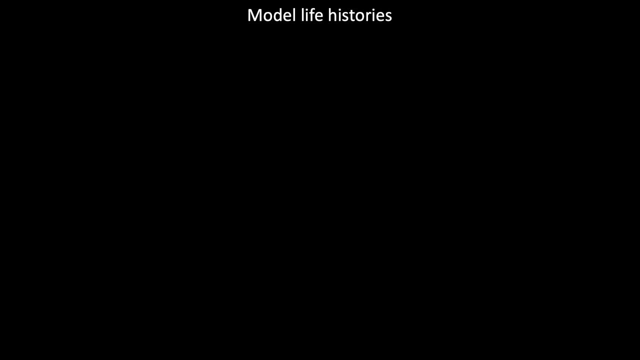 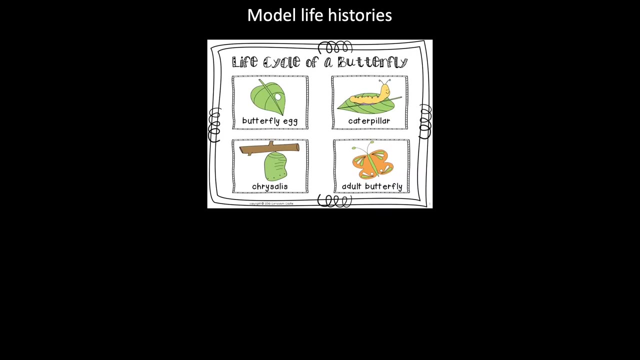 into a third category that we can call model life histories and the life history. i know that i've used that term earlier, but what it is is it's more than just the life cycle. many of you probably learned the life cycle of a butterfly when you were in. 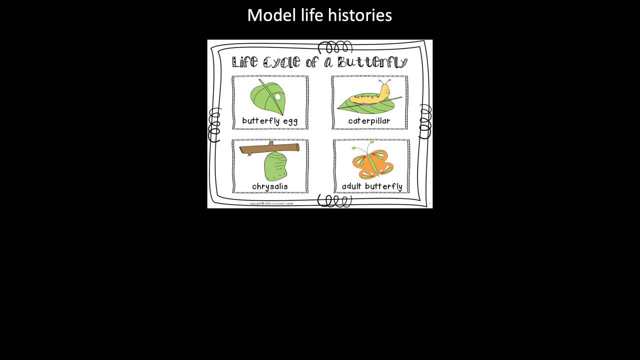 elementary school. and these organisms, as you may remember, have an egg that's deposited by the butterfly on a leaf, turns into a caterpillar that gathers a lot of food, before turning into a chrysalis or a pupa, and then, within that chrysalis, there is metamorphosis to the adult. 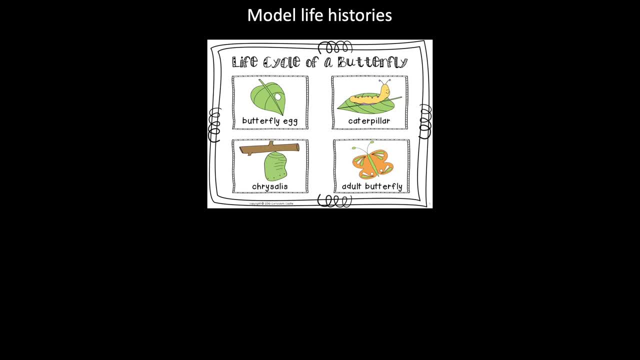 butterfly in marine invertebrates. there are a few organisms, such as the purple sea urchin, that are used as model organisms for early development, but the full scope of the organism's life is not considered by those researchers. most model organisms are direct developers without a larval form. marine invertebrates are not monophyletic. 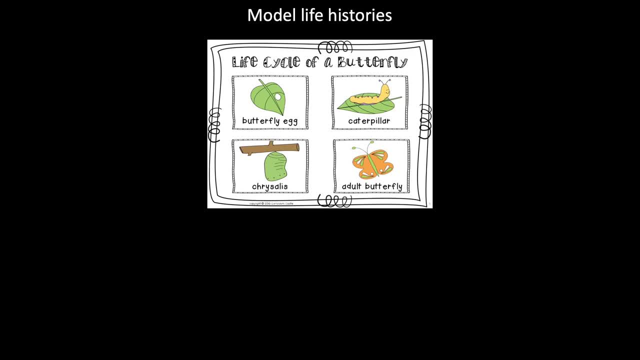 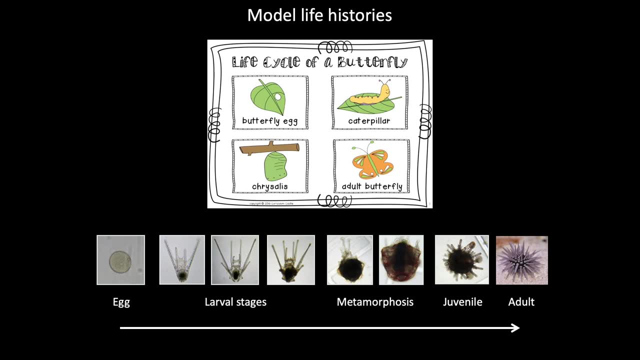 most of these organisms develop indirectly. they pass through one or more distinctive larval phases, and the name life history then suggests that comparisons at this level are made across the temporal sequence of the organism, in addition to those that are made within or across clades. so in the case of the chrysalis, there are a few organisms that are made within or across the. 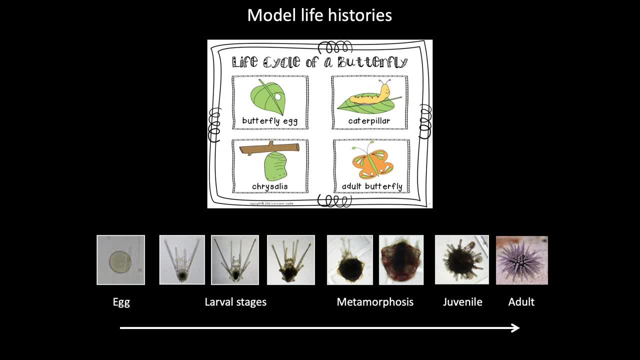 temporal sequence of the organism, in addition to those that are made within or across clades. in the case of the sea urchin, there is an egg, there are a series of subsequent larval stages, there's metamorphosis to a juvenile and then, ultimately, to an adult. this category of a model 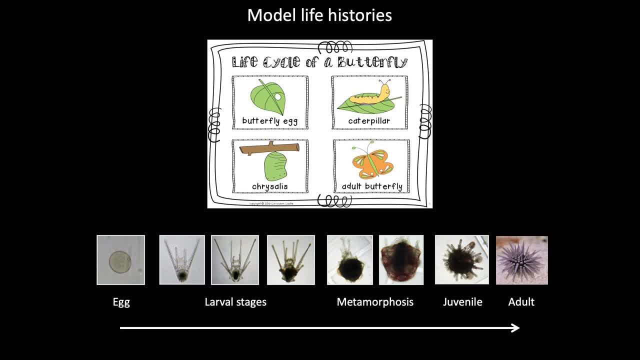 life history provides for the recognition of very novel kinds of representation, such as marine invertebrate larvae acting as surrogate models of ocean environments under changing climatic conditions. so we can use these model life histories to tease apart the way that the organisms interact with their environments and also how those different or changing. 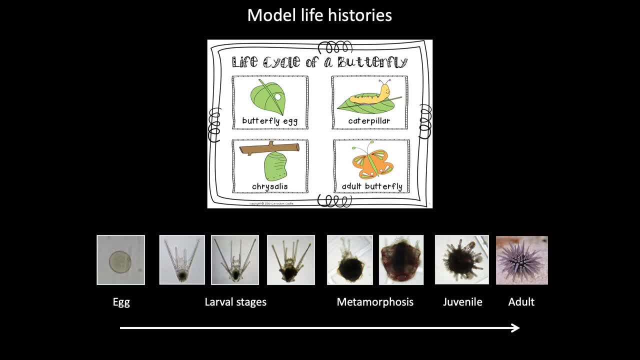 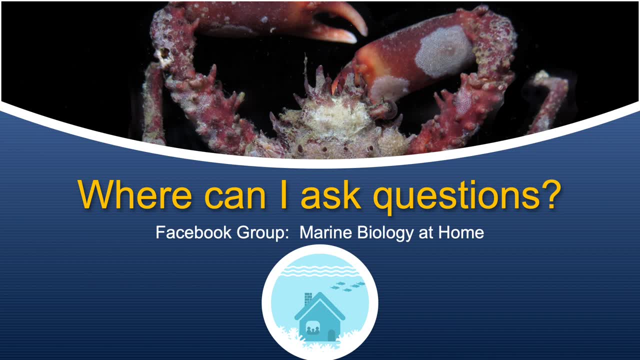 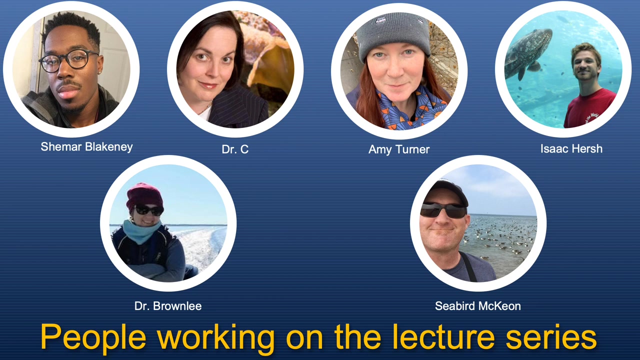 environments ultimately lead to differences in the development of organisms. if you're really interested in these topics, you're certainly welcome to to contact me. you can also ask questions to our facebook group, which is marine biology at home, and i encourage you to to be in touch. some of the different people working on the lecture series have been introduced. 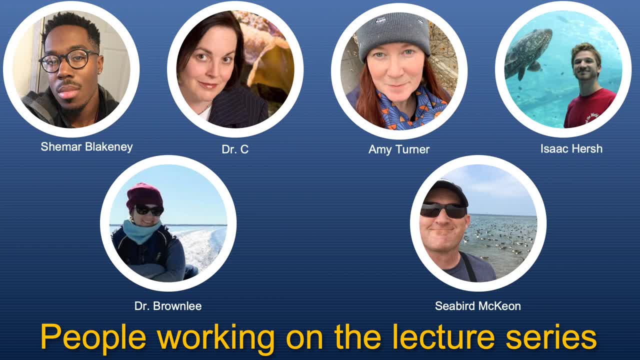 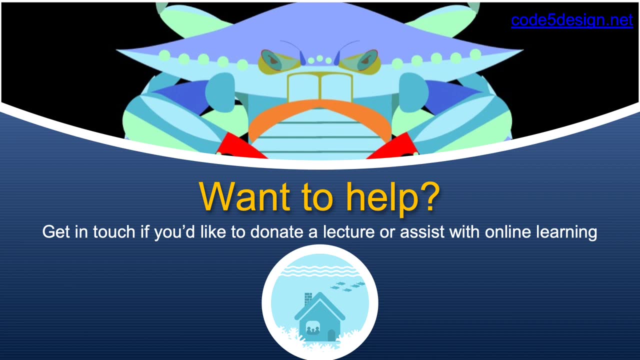 in previous lectures and i'll just show their pictures again here and you can contact seabird mckeon if you have questions specifically about the lecture series and if you want to help, feel free to get in touch. if you'd like to donate a lecture or to the seabird mckeon website, you can find me on the seabird mckeon website. 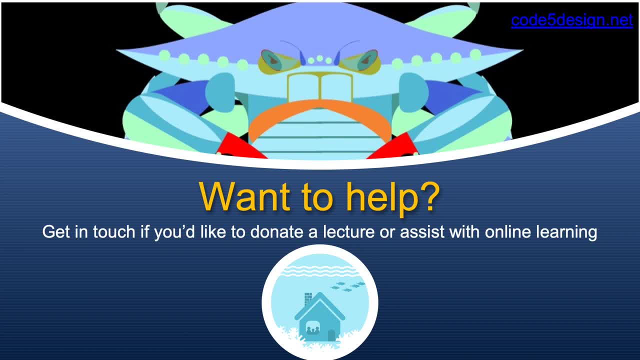 or if you'd like to assist with online learning. we hope to hear from you. thanks a lot.